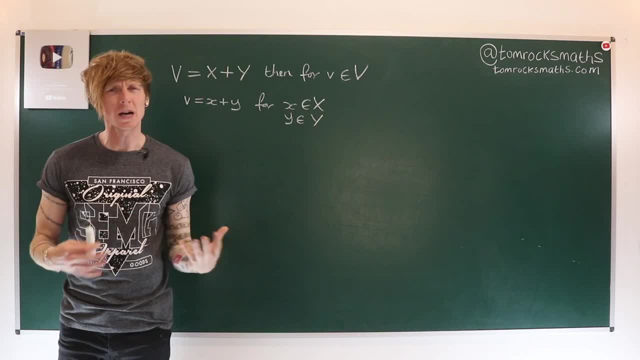 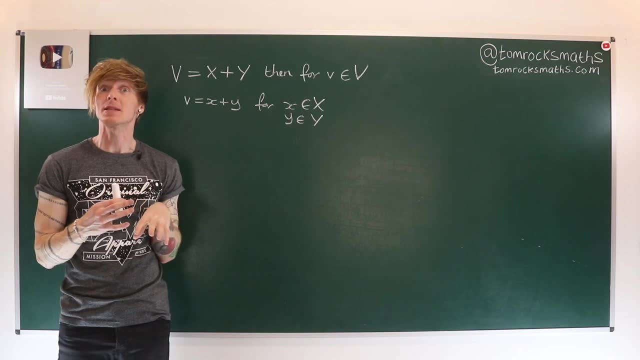 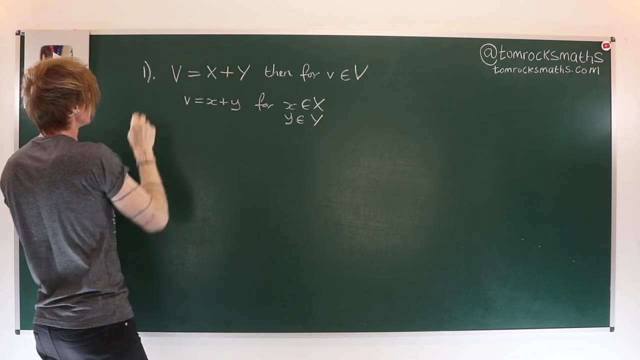 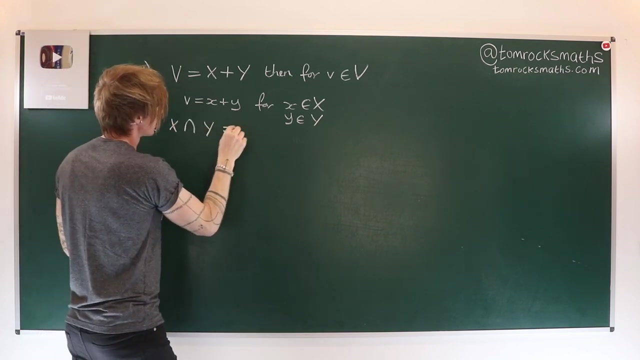 coming from the subspace. y. The direct sum of two vector spaces takes this concept a little further by insisting that the two vector spaces do not overlap. So we additionally, as well as this condition here for a direct sum, we additionally require that x intersect. y is only the zero. 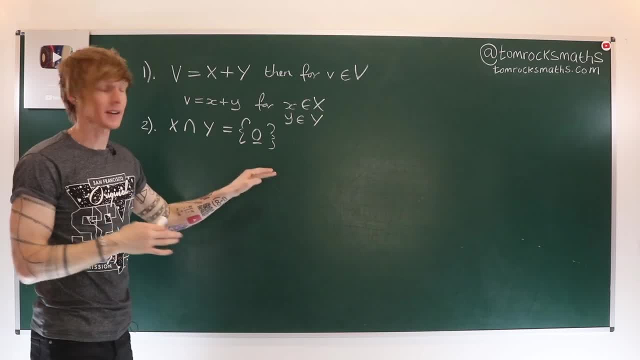 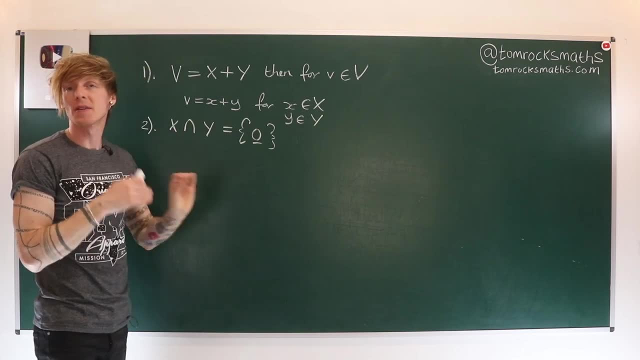 vector, And of course we have to have the zero vector in both x and y in order for them to be valid subspaces, but that is the only way to get the direct sum of two vector spaces, The only thing that they're allowed to share, And the formal definition is therefore to say: 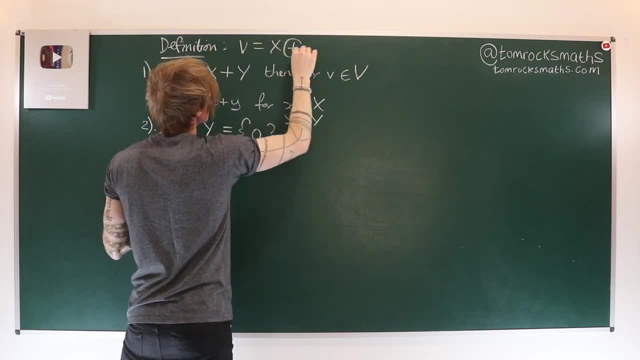 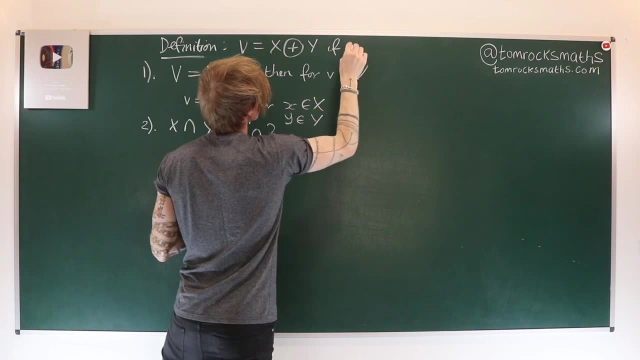 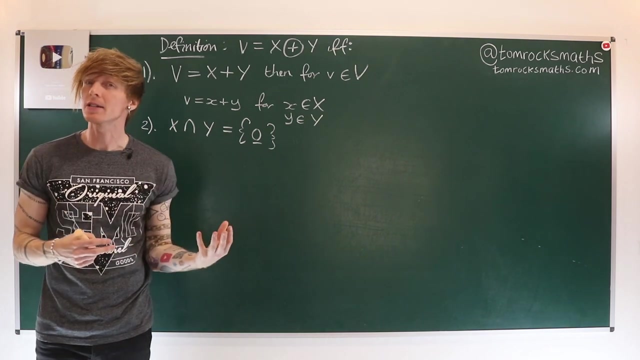 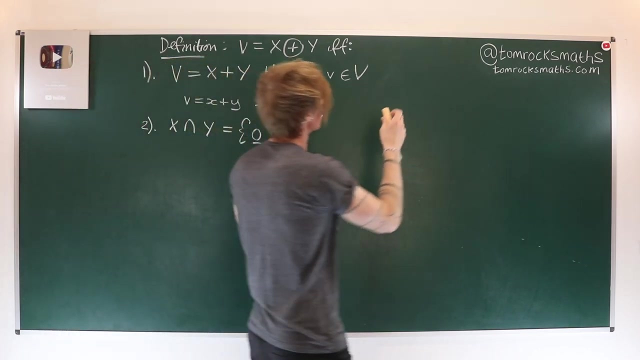 v equals x plus, with a circle around it to indicate direct sum y, if, and only if, the following two conditions are satisfied: Another alternative but very useful definition of a direct sum is the following. So let's call this alternative or equivalent definition. We can say that v is equal to x direct sum y. 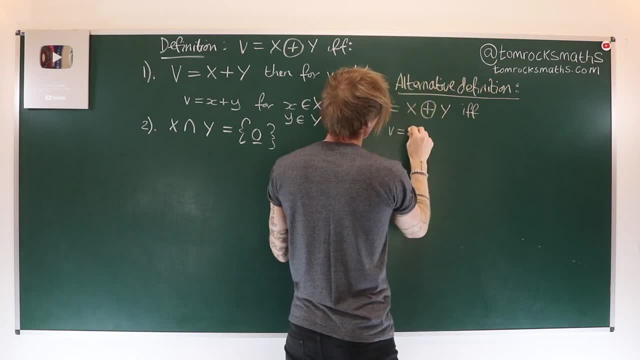 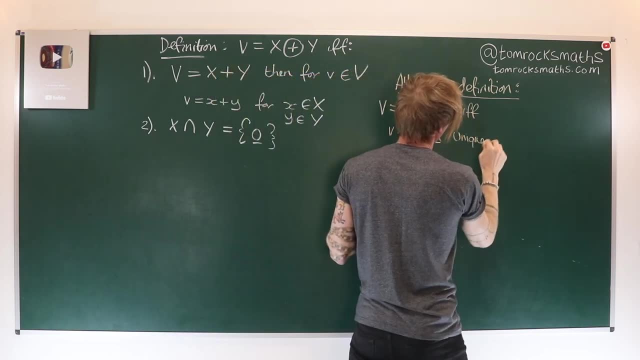 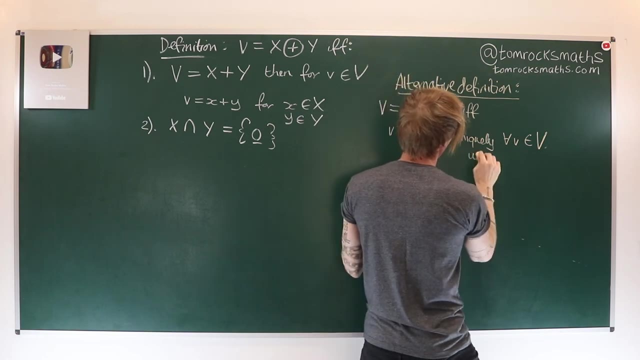 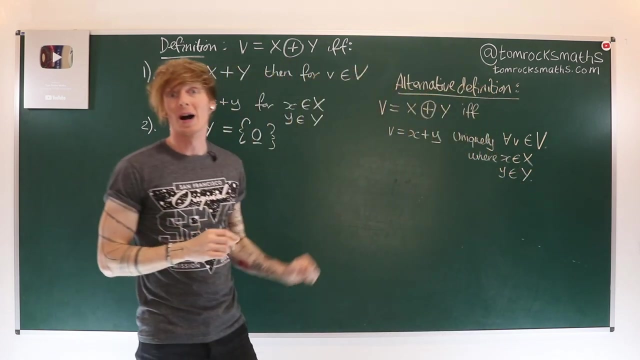 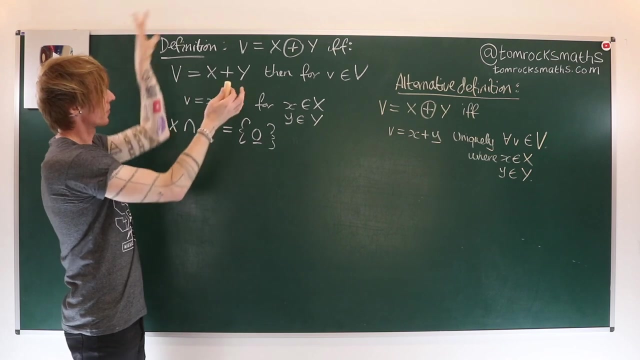 if, and only if, v is equal to lowercase x plus lowercase y, uniquely for all vectors v in our larger space v, where again x comes from x and lowercase y comes from the space y. So the key difference here between these two alternative but equivalent definitions is in the first one we have the intersection being zero. This is our formal mathematical. 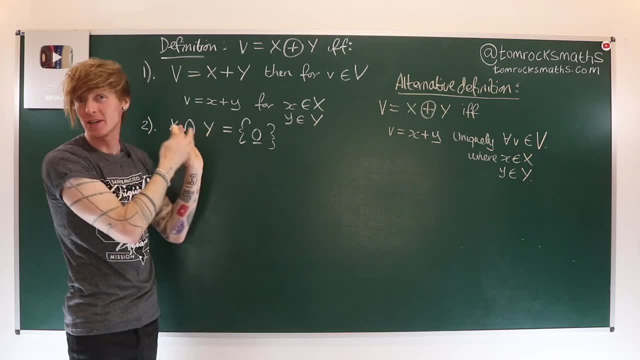 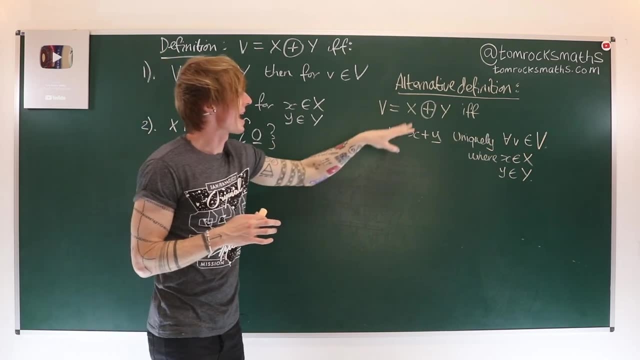 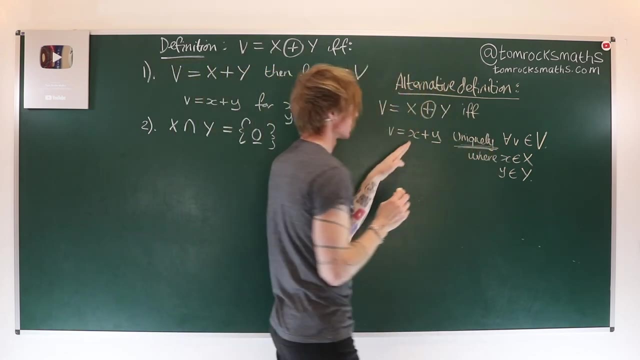 definition and the one I'm going to use as our standard definition, And I'm claiming that this is in fact, equivalent to this alternative definition, where every vector v in the larger space can be written uniquely as a sum of x plus y for some part x in the space x and some part y in the space y. 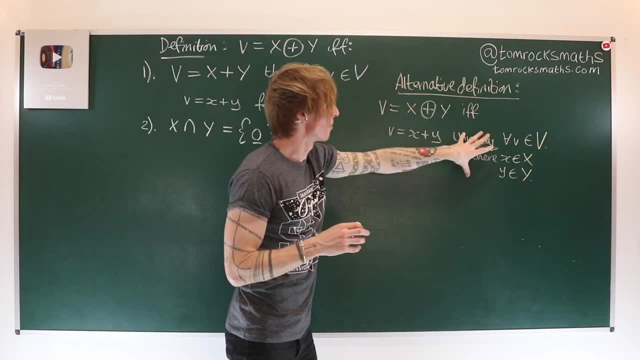 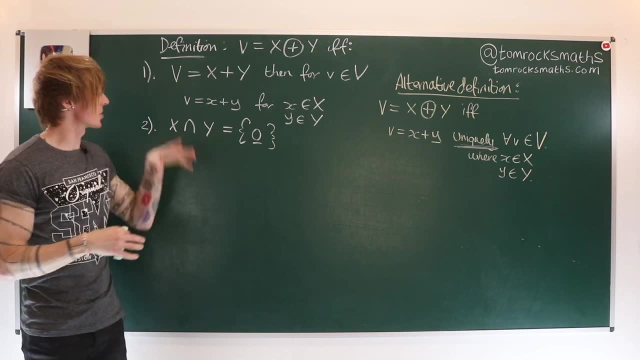 So the key thing here is going to be this uniqueness, and we're going to have to show that these two are in fact equivalent by doing a proof First. let's suppose both conditions- one and two, are same, So proof- and this is going to be from the left, assuming this is true- show the alternative definition also holds. 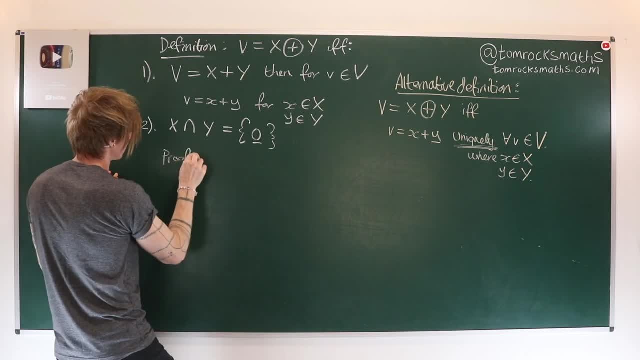 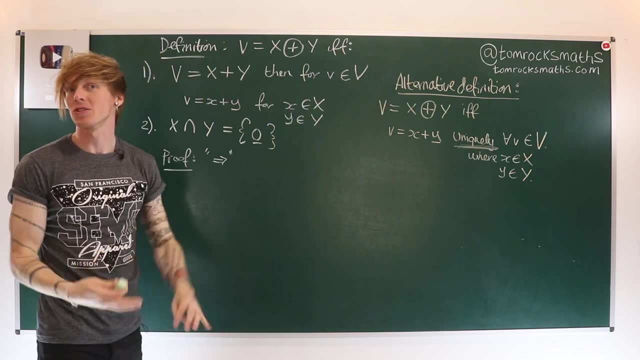 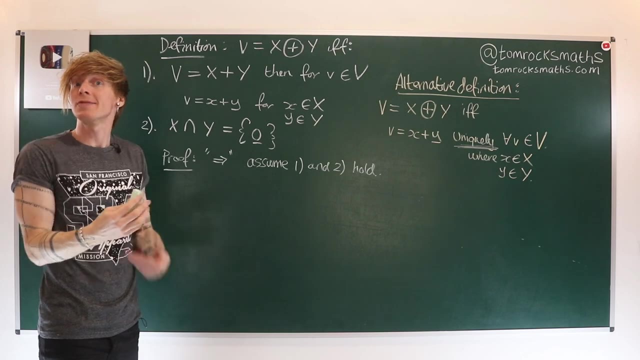 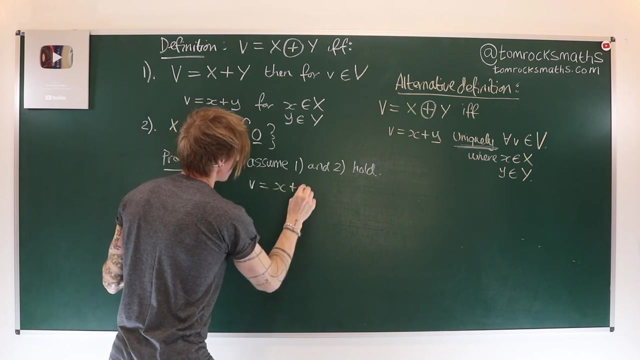 So proof- and this is going to be from the left, assuming this is true- show. the alternative definition also holds. Okay, so we assume one and two hold. and let's suppose we have two different ways of writing out a vector, v. So let's suppose that v is x plus y. 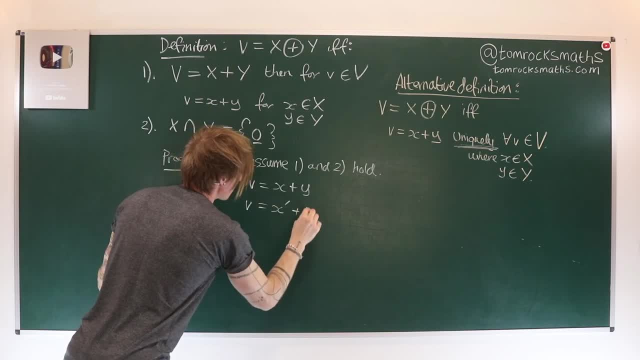 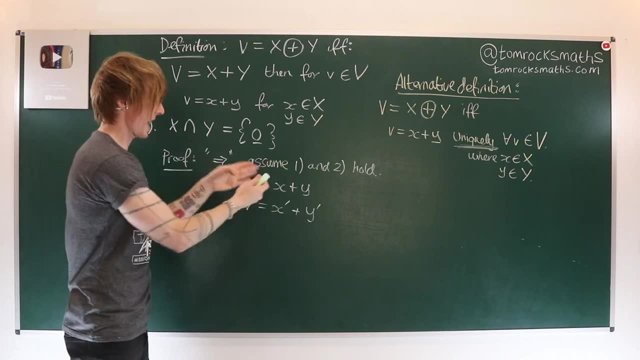 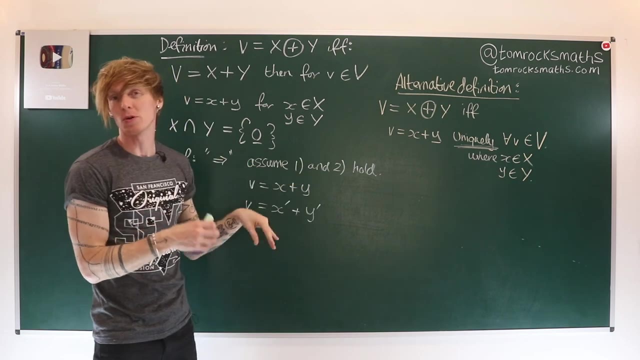 and it is also equal to x prime plus y prime, and our goal here is to show that in fact, these are the same. so therefore, we need x to be equal to x prime, because that is the piece that belongs to the space x, and we want to show that y is equal to y prime. ie, we started by assuming. 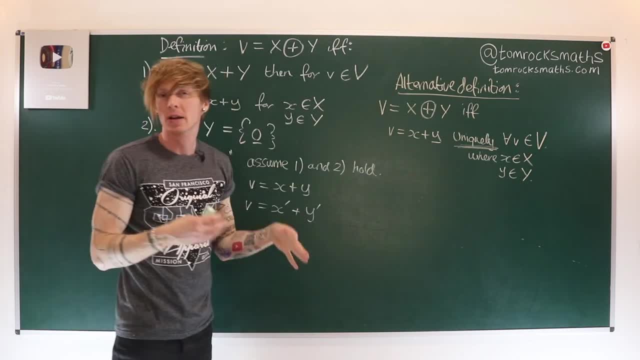 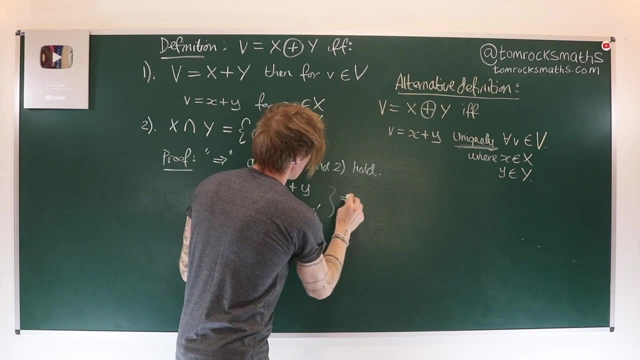 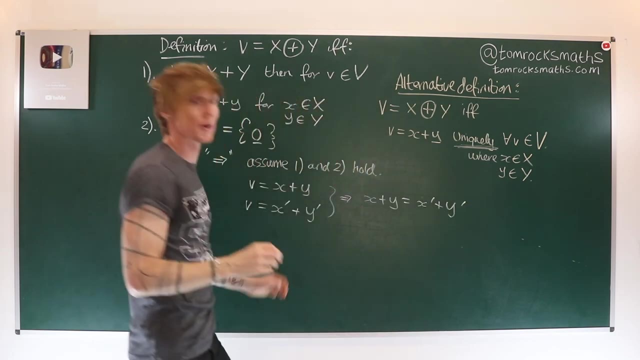 that there were two different ways and then showed in fact they are unique. So, because both of these are the same, we can rewrite this therefore and say so: therefore, x plus y is equal to x prime plus y prime, because both of them are v. and then, if we group the x terms, we've then got x minus x prime. 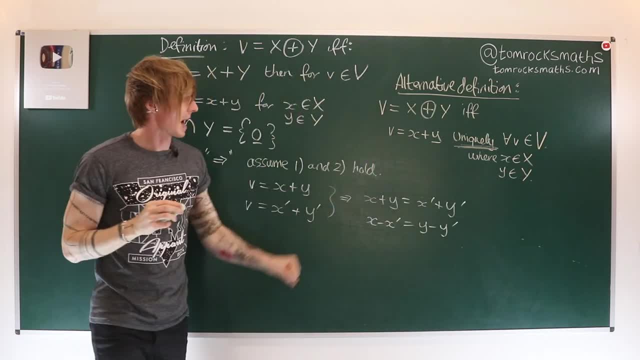 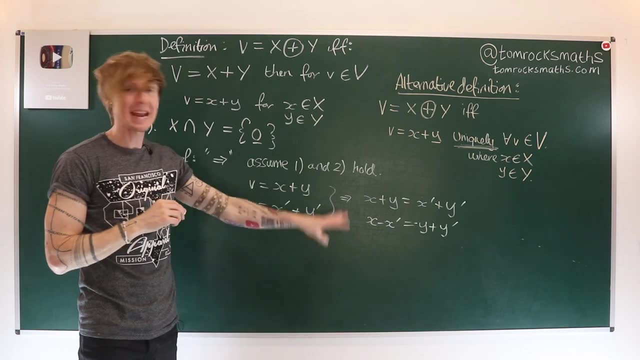 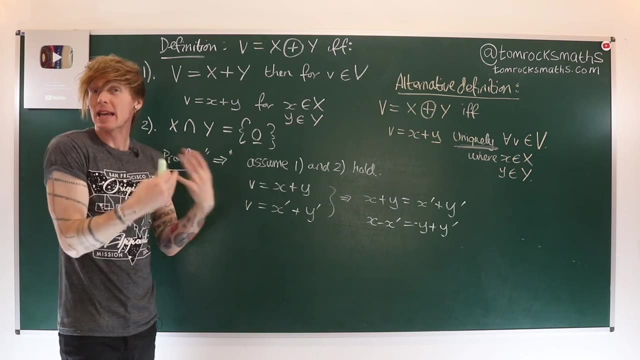 is equal to y minus y, prime grouping the x's on the left- and it's actually going to be minus plus- and the y's on the right. Now both belong to our space X. Our space X is a subspace, so that means any two. 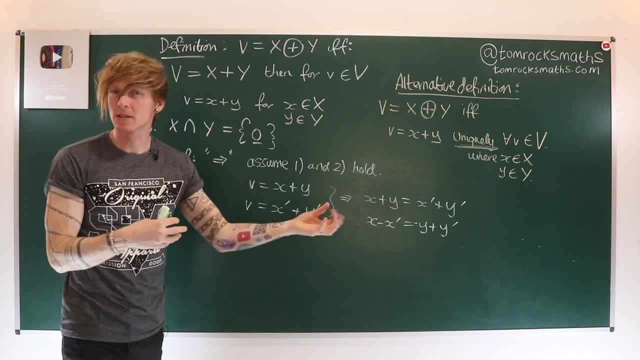 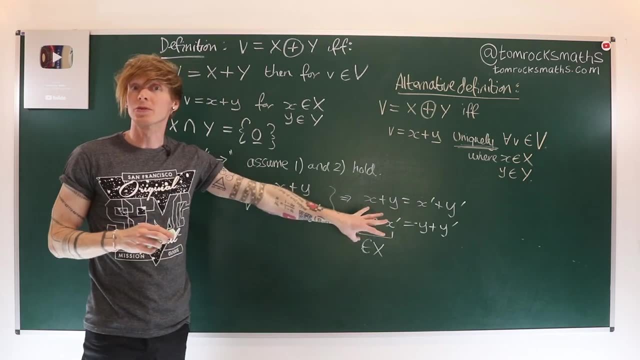 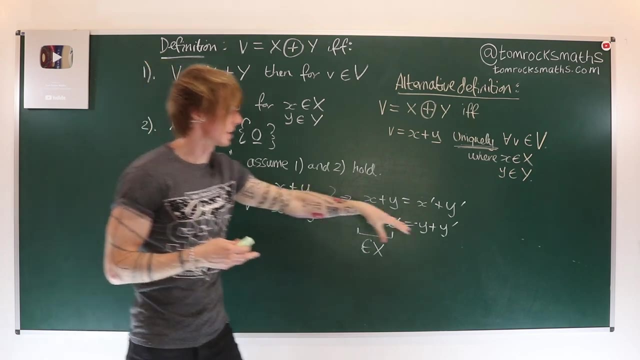 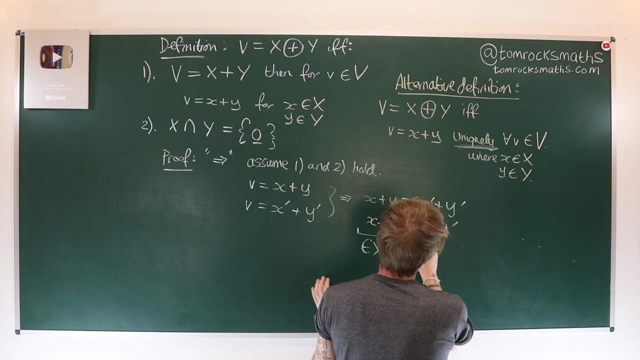 vectors in it. when you add them together you get something else in the space. So this definitely belongs to X and it's equal to this thing on the right. but again we have two pieces, Y and Y prime. We have a linear combination of those two pieces and the two pieces belong to Y, So the linear combination also belongs. 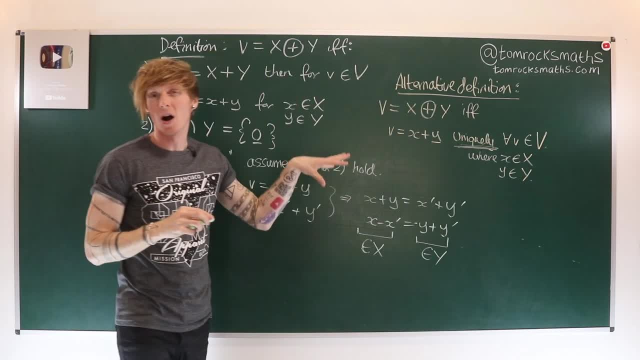 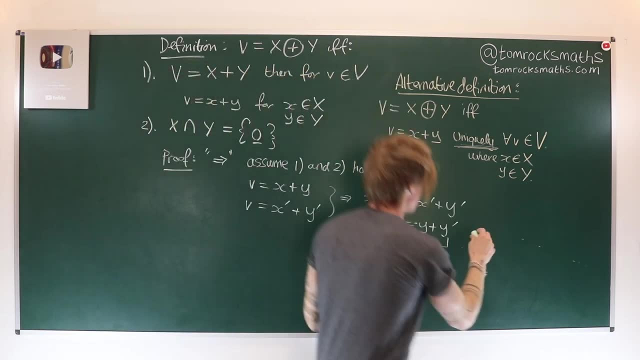 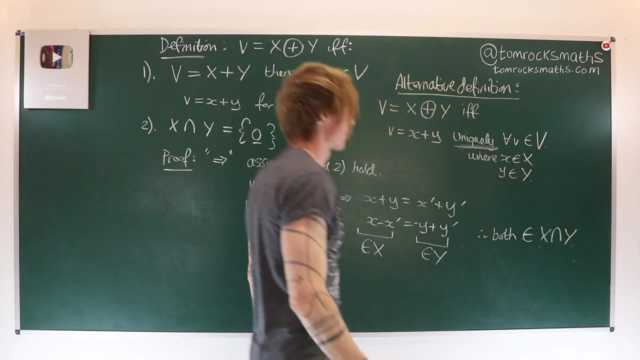 to Y and once again, these two are equal. so we have something in X, equal to something in Y. therefore, both of them must- in fact both must- belong to X, intersect Y. However, we've got from number two up here, which we have assumed to be true. 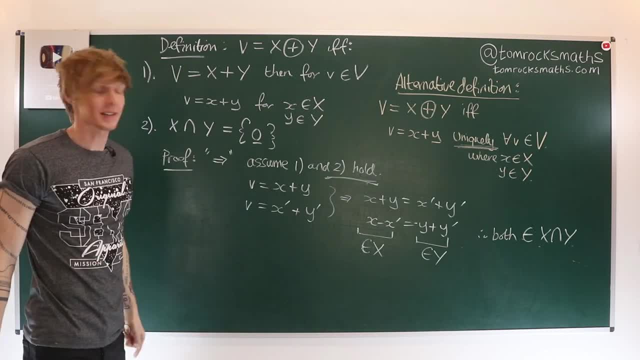 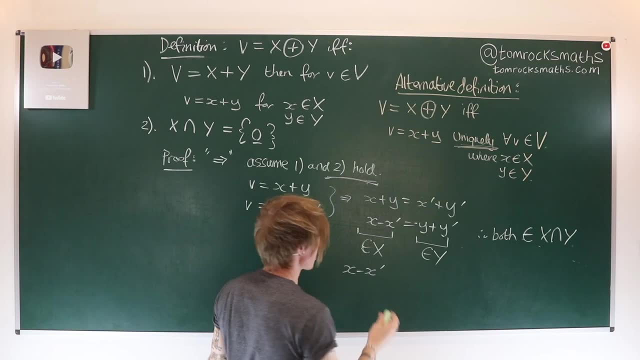 The intersection is just the zero vector, so if the left-hand side, so X minus X prime, belongs to the intersection, so therefore is equal to zero, and Y minus Y prime or minus Y plus Y prime is also in the intersection, which is also equal to zero. so that's just equivalent to saying that X is equal to X prime, Y is equal to. 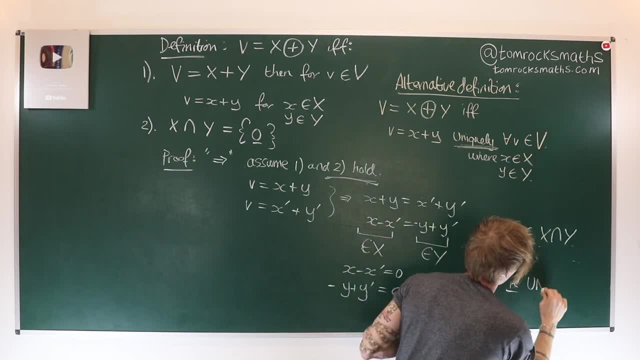 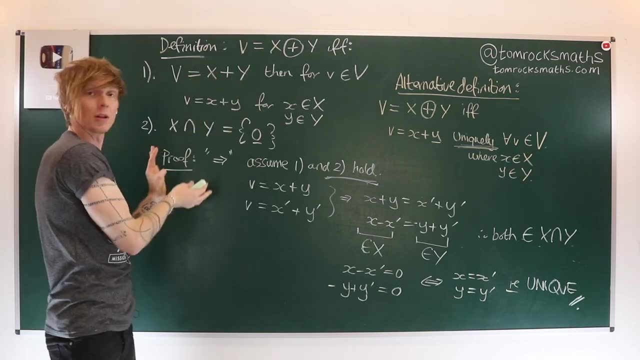 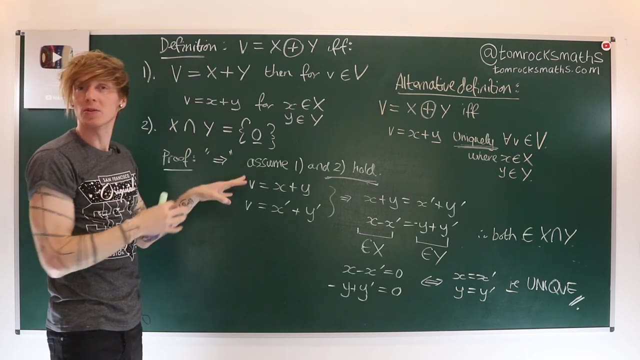 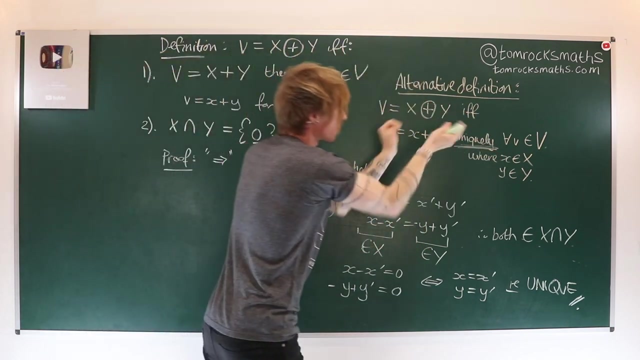 Y prime ie unique. So, starting from the formal definition, the mathematical definition that I'm using on the left of the board, we assumed conditions one and two held and we were able to show that the uniqueness property will actually follow. so therefore, this definition implies the alternative To complete the proof we of 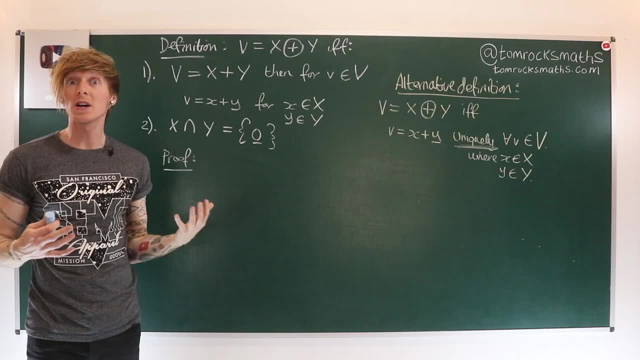 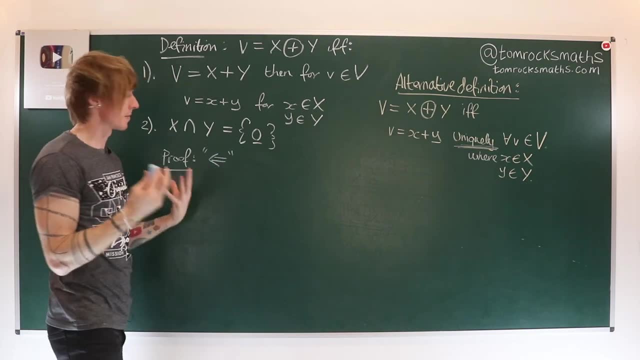 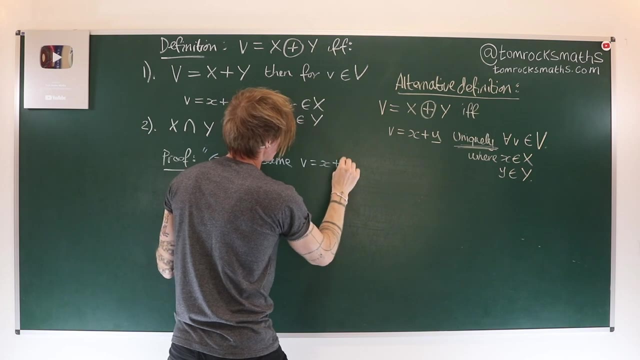 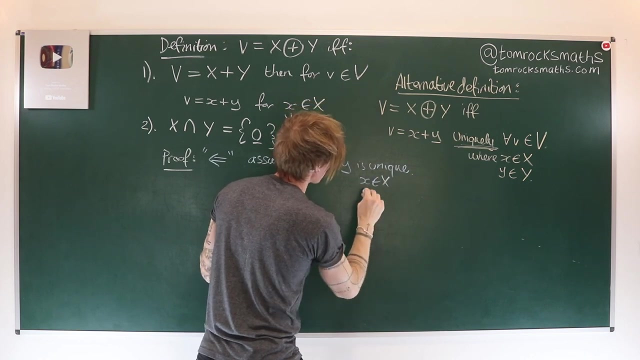 course have to go back in the opposite direction. For the reverse. we now need to go from the right-hand side of the board to the left, Back to the left. so we are going to begin by assuming the uniqueness. So assume V is equal to X plus Y is unique, and this is of course for X in capital X. 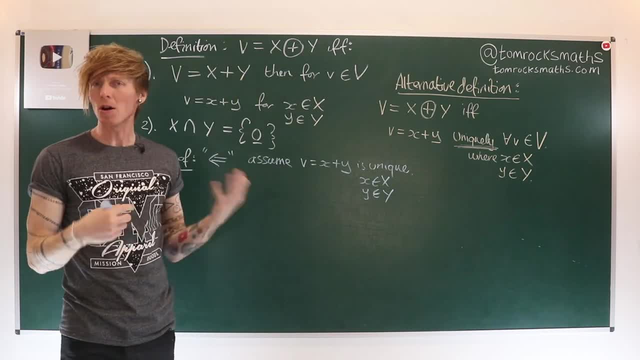 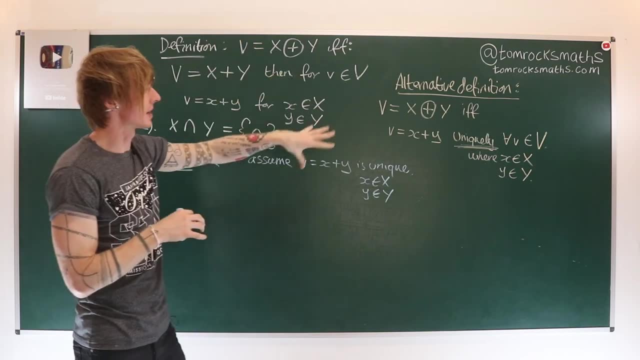 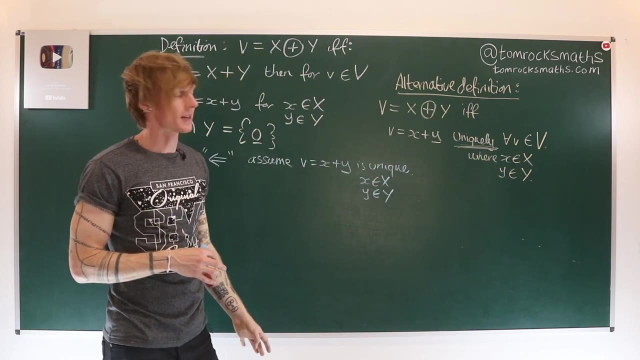 and Y in capital Y. Now, our goal here is in fact to show condition two to be true, because condition one is automatically satisfied precisely by the alternative definition. this tells us that for every V in our larger vector space V, we can write it uniquely in these two pieces, and therefore that gives us number one. 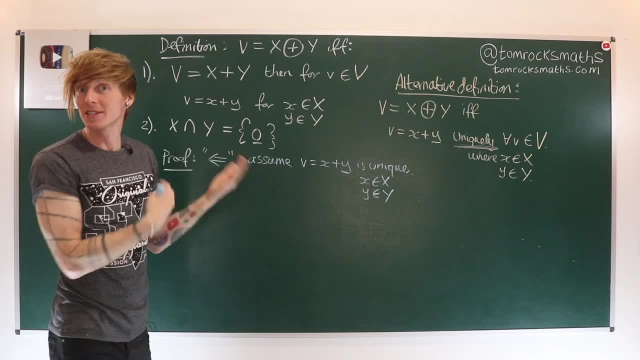 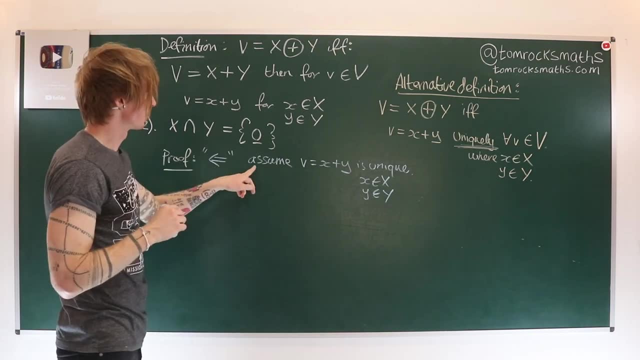 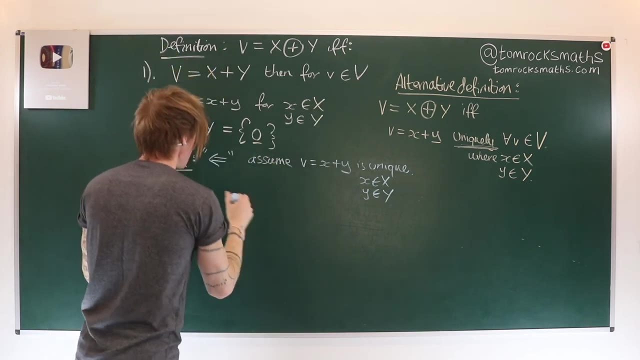 So we just need to show that the intersection is equal to zero and then we have our full proof and we have our equivalence between the two definitions. So therefore, let's assume that this V is in fact in the intersection. so assume V is. this is unique. that's from there. and let 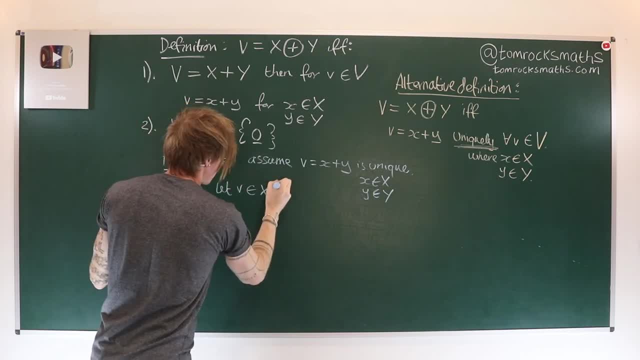 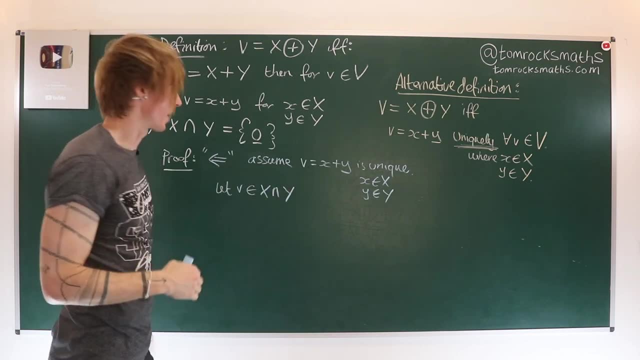 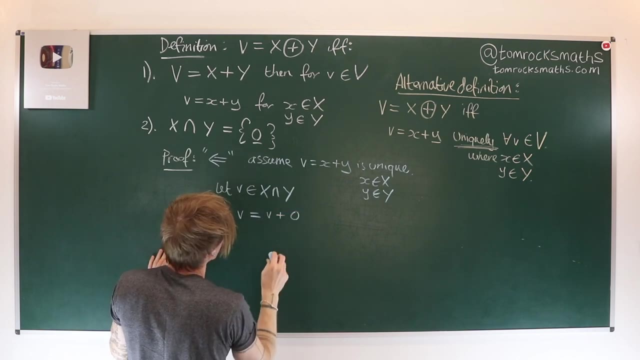 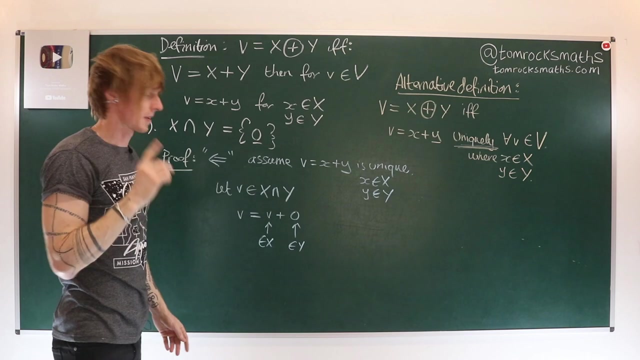 this v actually belong to the intersection Now, because it's in both x and y. it's still in v, the large space. so we can say: v is therefore equal to v plus 0, where this one belongs to x and this one belongs to capital Y. But I can. 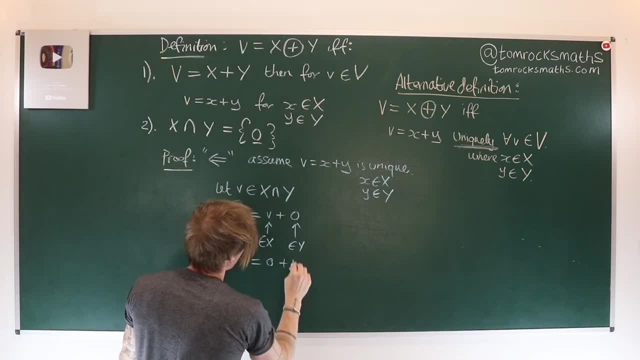 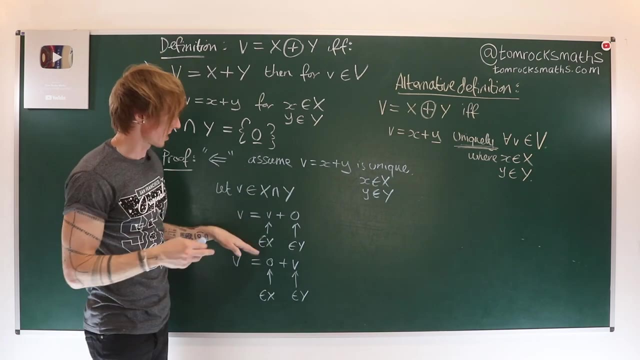 also rewrite that as 0 plus v, where 0 belongs to capital X because it's a subspace, so it has to, and v belongs to y because we assumed v was in the intersection. So I've actually got two ways of writing out the same vector: v. 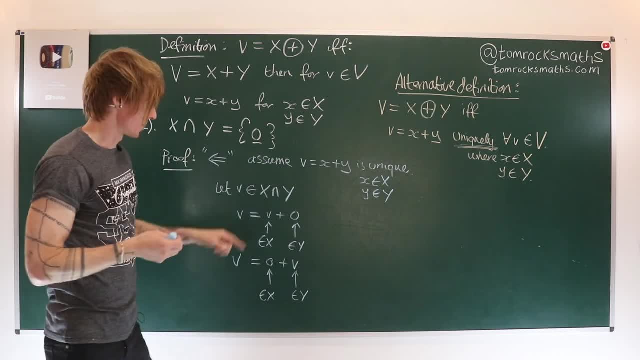 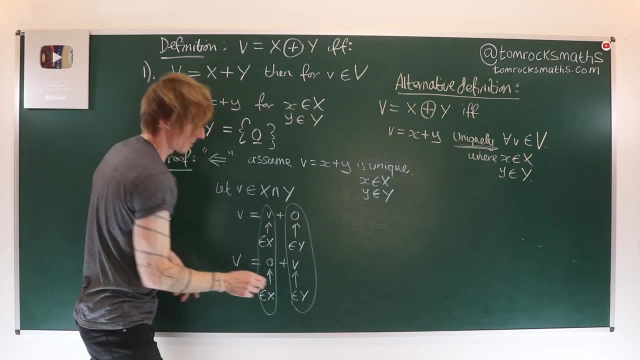 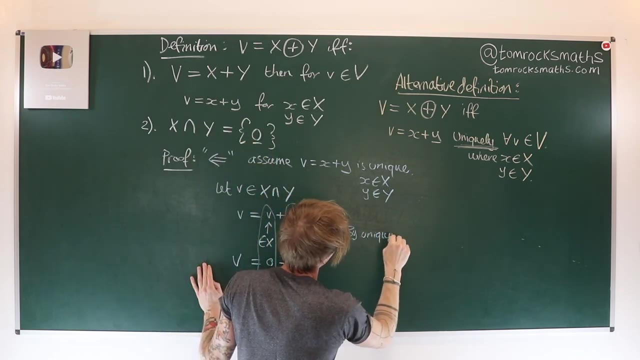 when v belongs to the intersection. So what that means, then, is these two pieces, in fact, must be equal and similarly here, but both of them give us the same result. So therefore, by the uniqueness property- and we did need that, but by the uniqueness- we can say that v 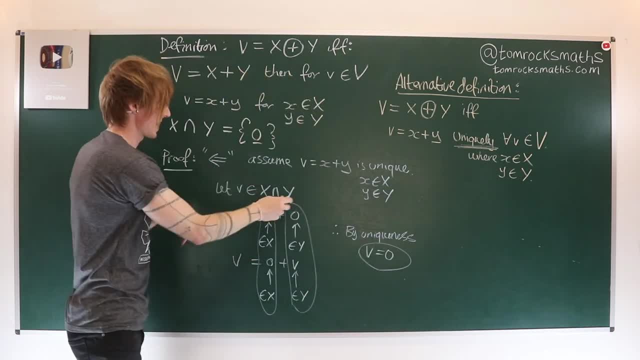 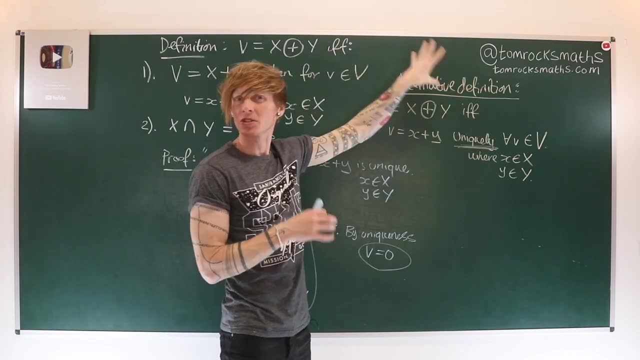 is in fact 0, ie any vector that's in the intersection is in fact 0 by uniqueness, and therefore the right-hand side definition, the alternative definition, is equivalent and the same as the one on the left. So that completes. 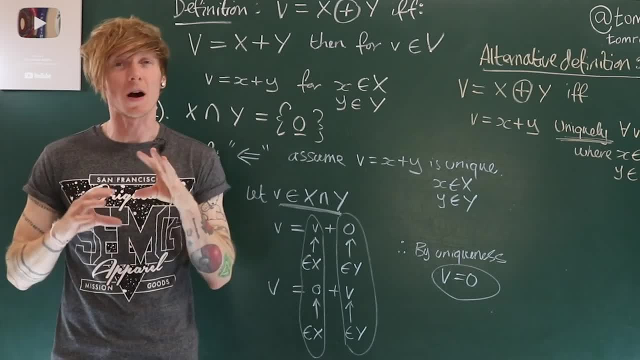 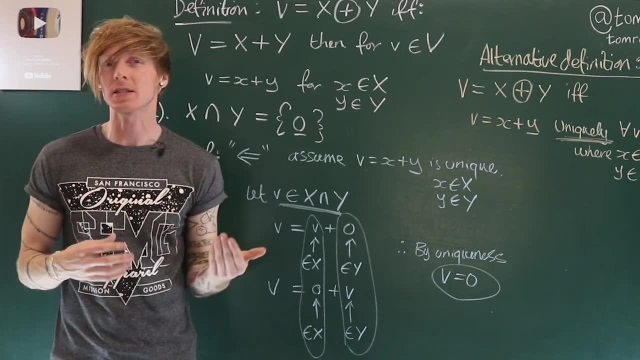 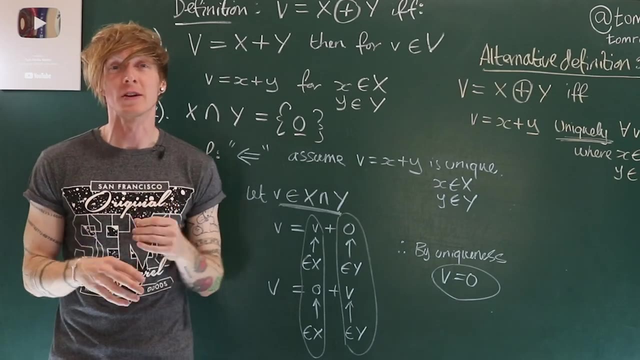 our proof that these two definitions of a direct sum are equivalent. However, if you'd like to see even more equivalent definitions for the direct sum, as well as an explanation about how a direct sum works in practice, then I recommend heading over to ProPrep an. 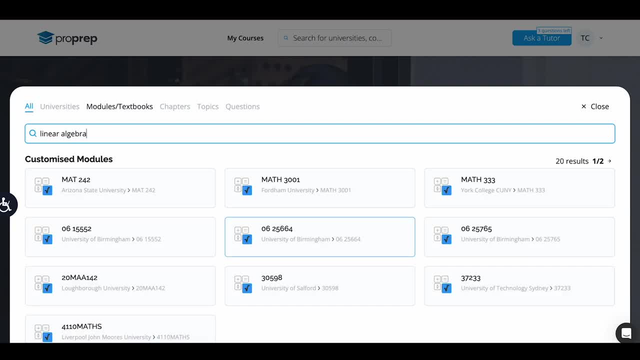 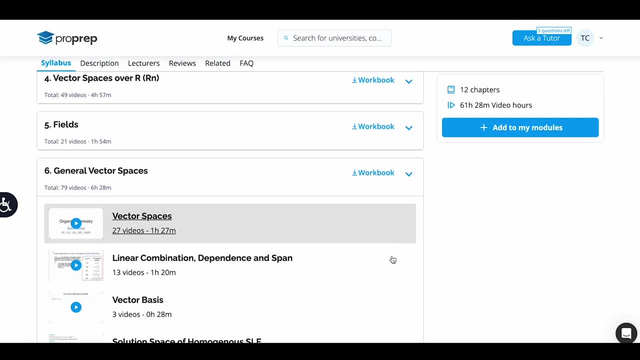 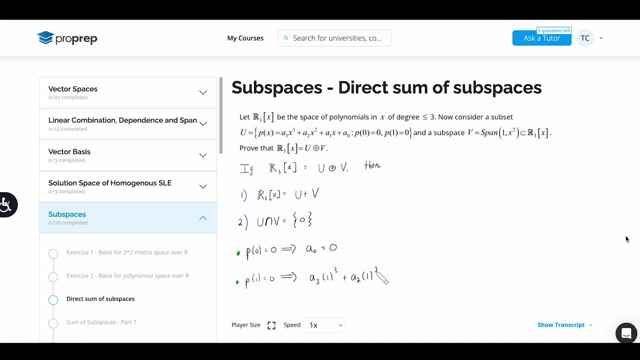 online resource which provides customized tutorials for students looking to improve their skills in stem-based subjects Under the general linear algebra course. you can find a section entitled subspace, which is a tutorial on subspaces, which contains four lecture videos exploring the topic of. 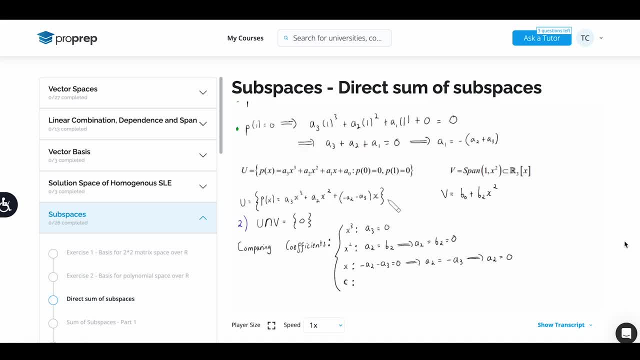 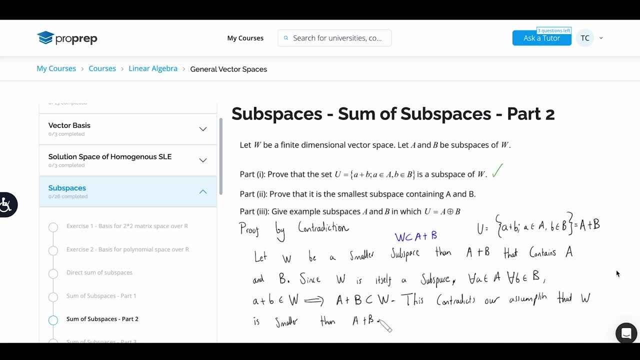 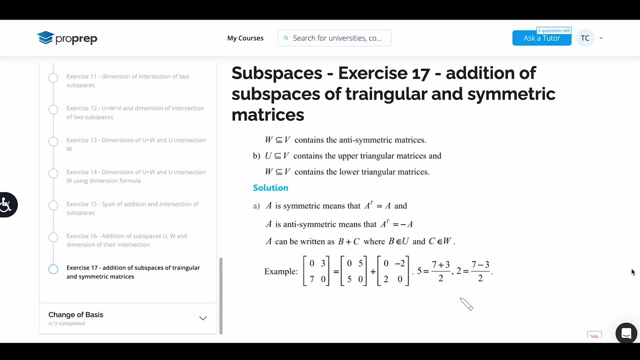 direct sums. They begin with some examples using polynomial vector spaces before progressing onto the more general case, like we've been looking at in the video so far. As usual with all topics on ProPrep, there are of course several exercises for you to try, with complete video solutions so you can check every. 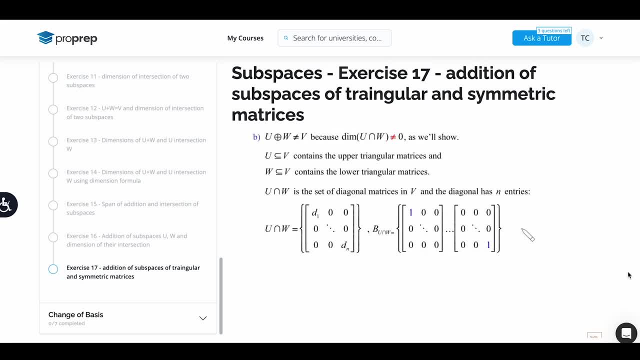 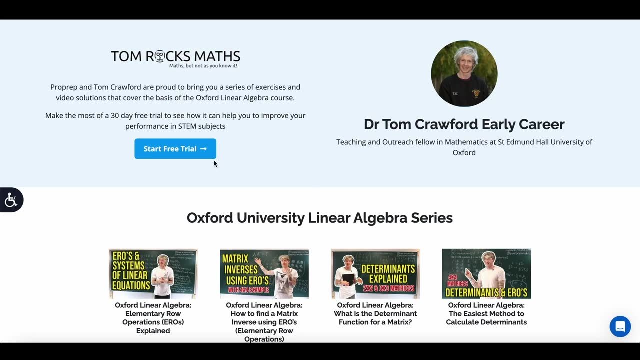 step of your working. One of the later exercises on triangular matrices is a particular favorite of mine, as it hints at the power of direct sums as a means of dividing up a larger vector space into smaller pieces. Try it out for yourself now, with a 30-day free trial, courtesy of Tom Rocks Maths: Just click. 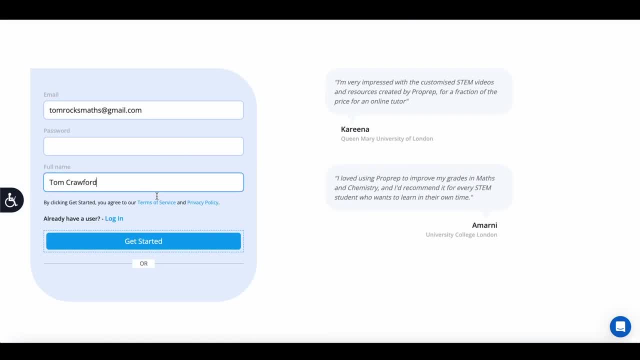 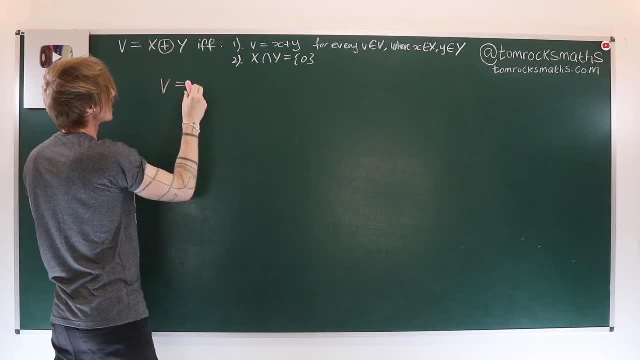 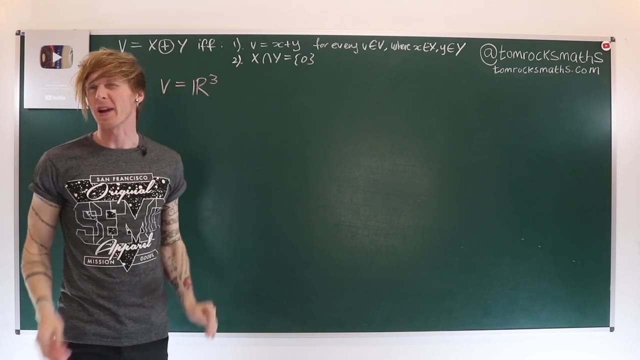 the link in the video description to sign up to ProPrep and get started right away. Time for some examples. So let's suppose that V is going to be R3, so three-dimensional coordinate space, x, y, z, the coordinate axes. And let's suppose we have a subspace X. and if you 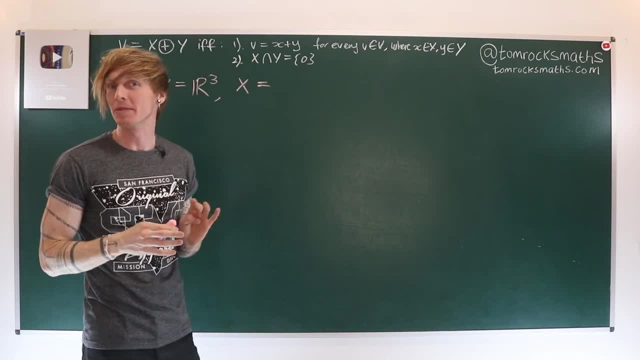 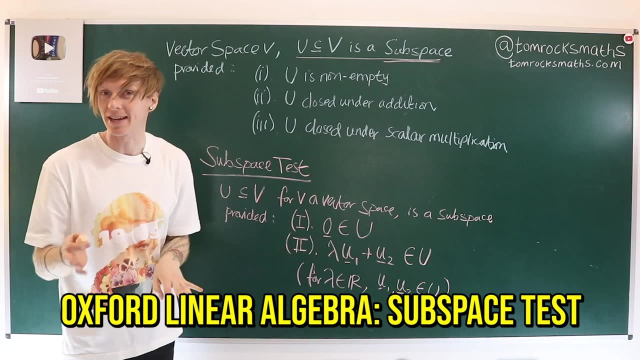 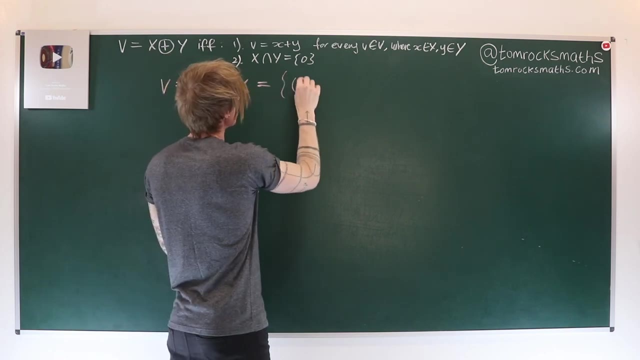 would like an exercise. you can check that what I'm about to write on the board is indeed a subspace by using the subspace test which is introduced a few videos previous in the Oxford linear algebra series. So let's take X to be equal to triples x, y, z, such that 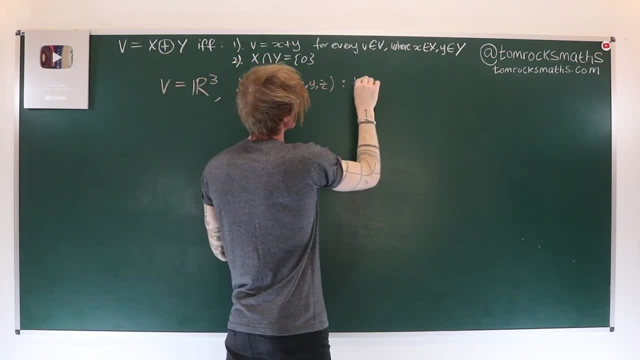 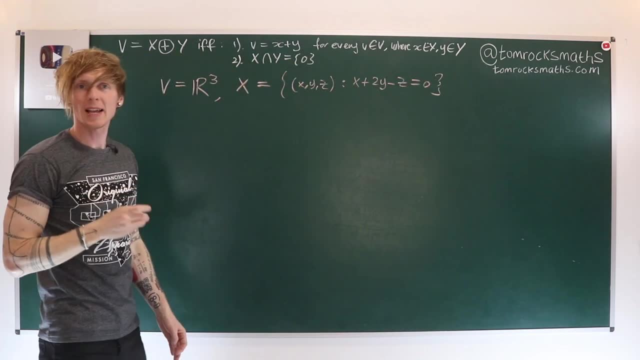 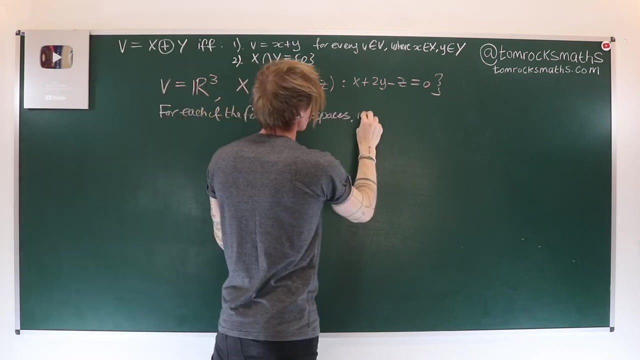 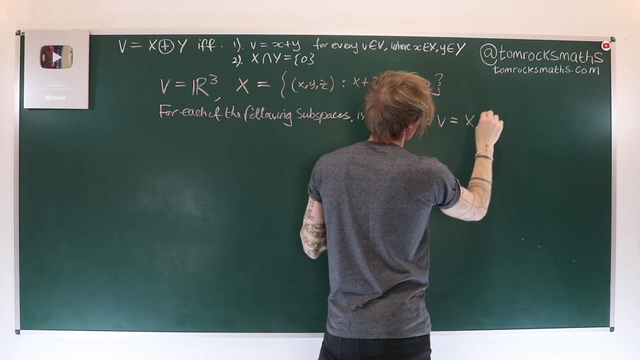 the following is true. So X plus 2y minus z must be equal to 0.. And what we would like to calculate or work out is for each of the following: Is it true that V is equal to X? direct sum y question mark. So I'm going to write out: 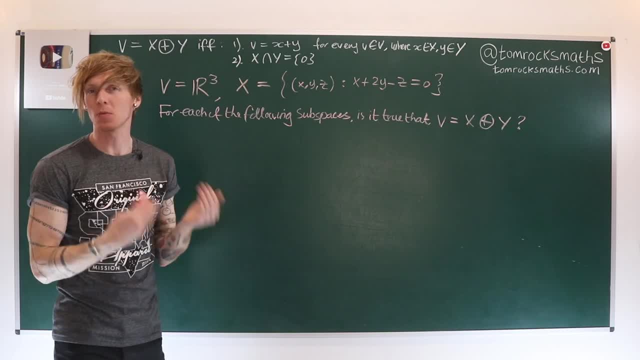 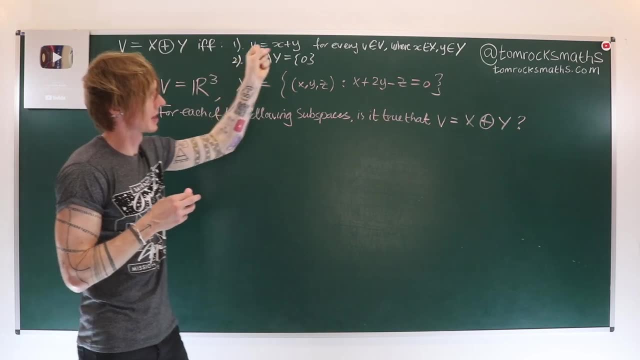 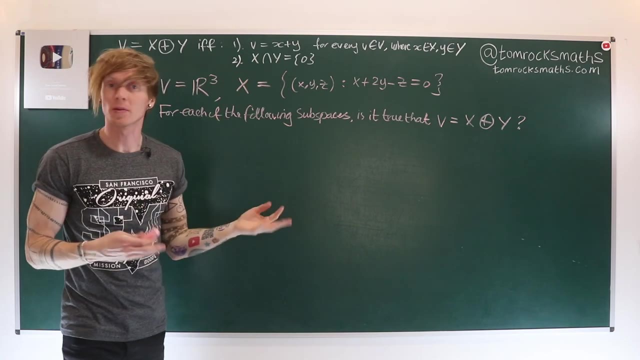 three different possible subspaces: y, and our task here is to work out if it's possible for V to be written as X, direct sum y. If it is, we're going to have to prove that is the case, Or if it isn't true, then we're going to have to give a. 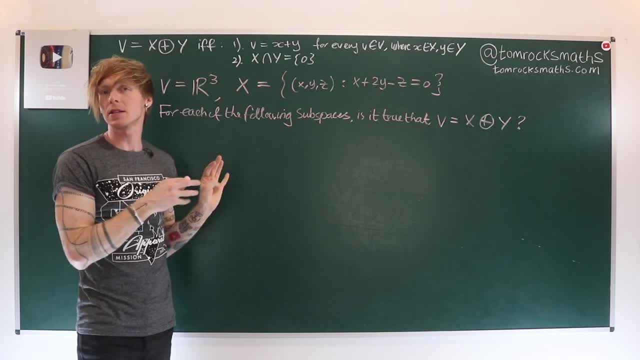 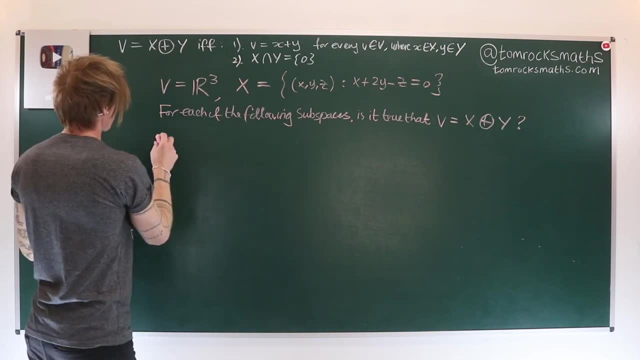 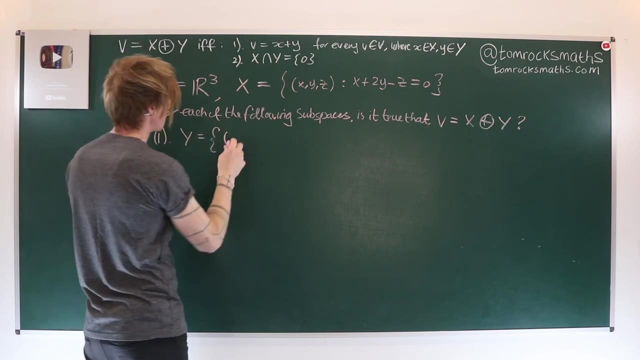 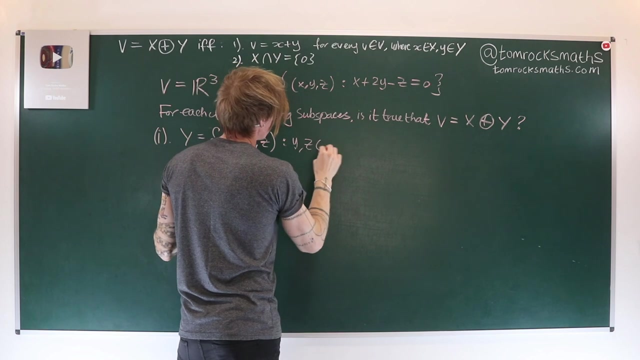 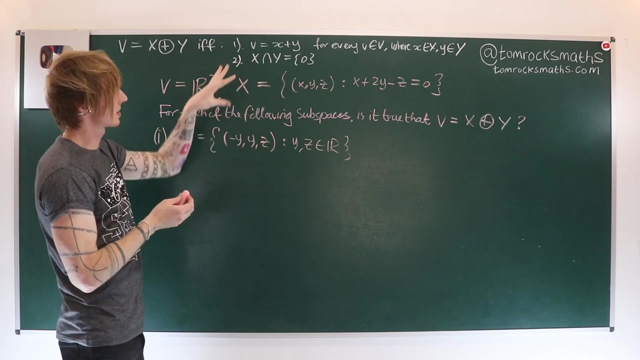 counter example and give a reason why the direct sum does not hold in that particular instance. For our first example, we will consider the following subspace: Y is equal to the set of triples or three vectors where we have minus y, y, z, where y and z can be any real number And we want to check: is it true that X? 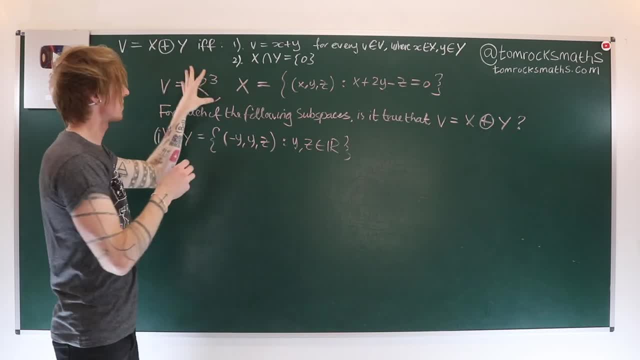 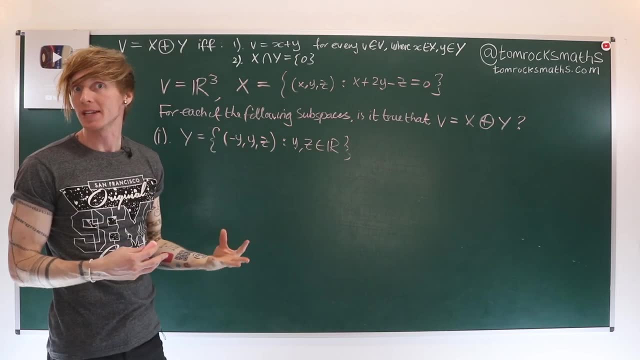 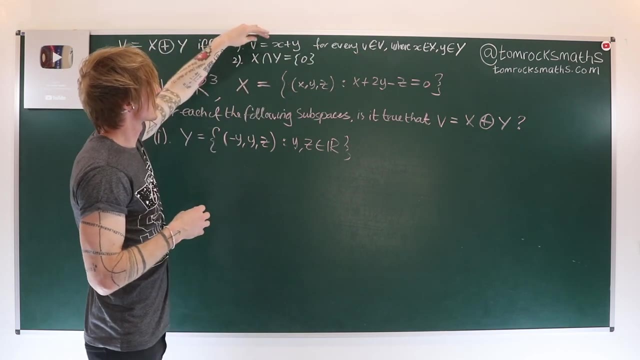 direct sum y is equal to the whole space V, which is R cubed. Now we have to check the both conditions of our definition of a direct sum are satisfied. so we need to check that for any vector in R3 we can rewrite it as something from X plus something from Y, and we have to. 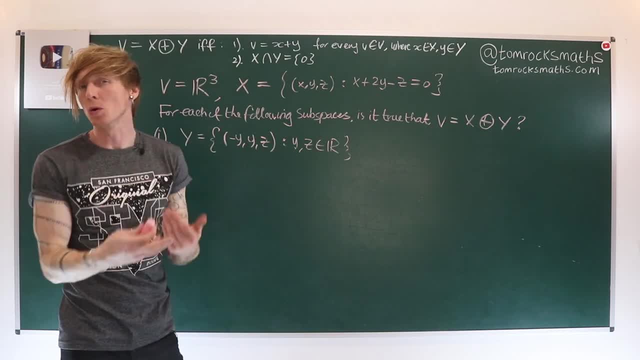 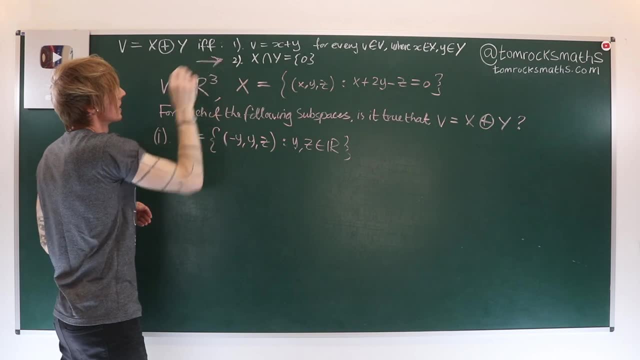 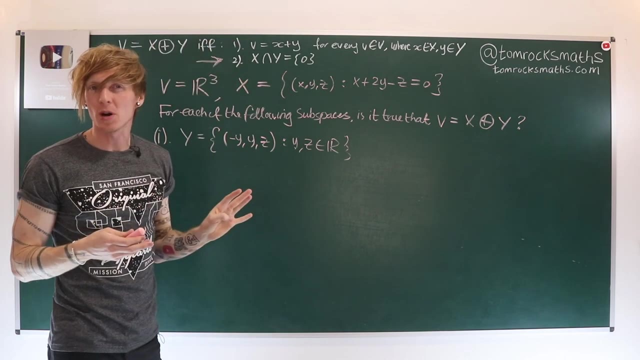 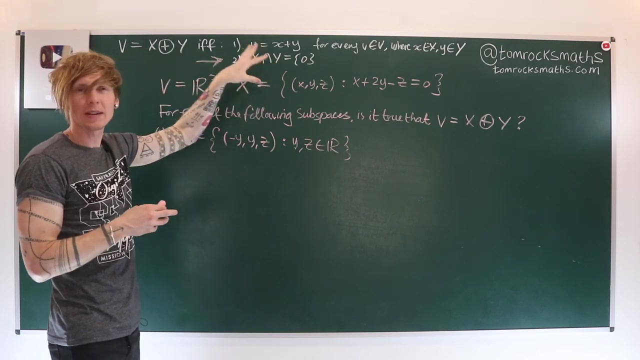 check that the intersection of our two subspaces only contains the zero vector. So this one is usually the best place to start, because it's quite an easy thing to check. This generally requires quite a bit of work in solving various systems of linear equations, as we'll see shortly, but checking the intersection is very 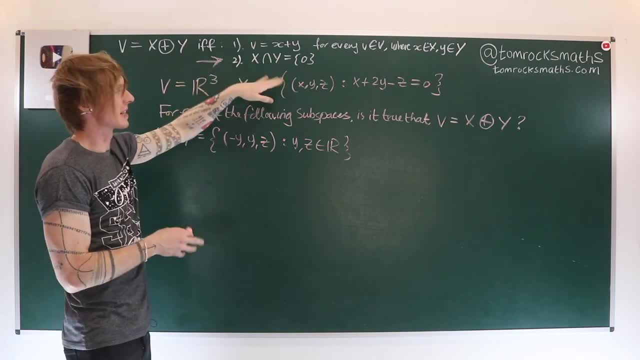 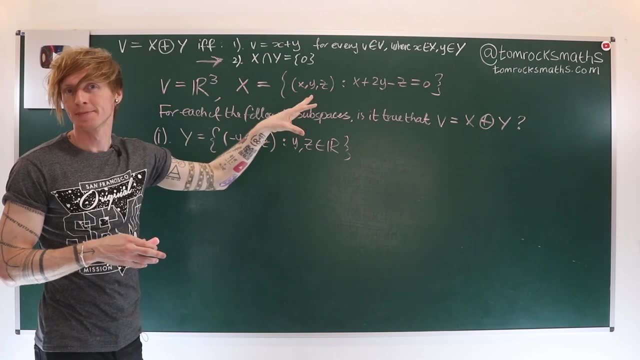 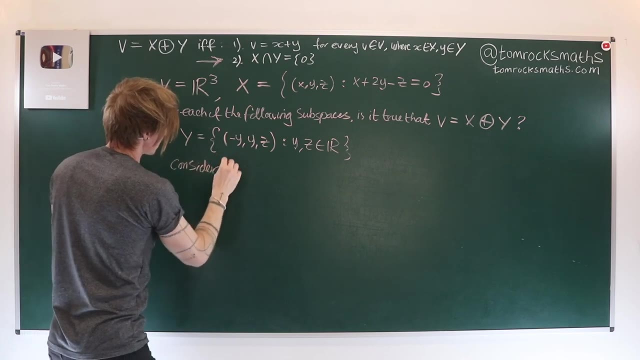 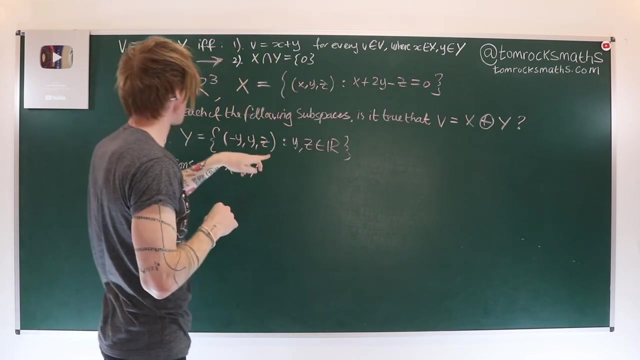 helpful at the beginning, because if we get something that isn't zero, we can immediately conclude that it is false. it is not a direct sum. So if we start with that, so we're going to consider the intersection. So any vector in both X and Y has to satisfy this equation and has to have 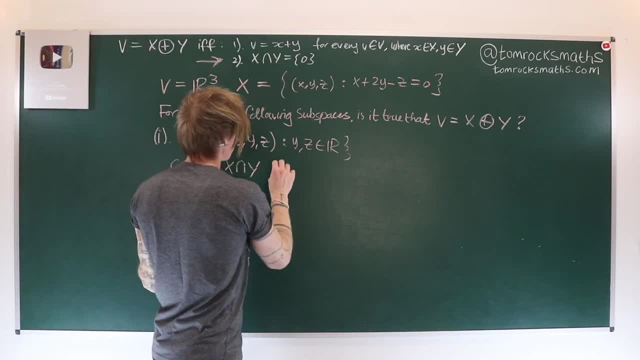 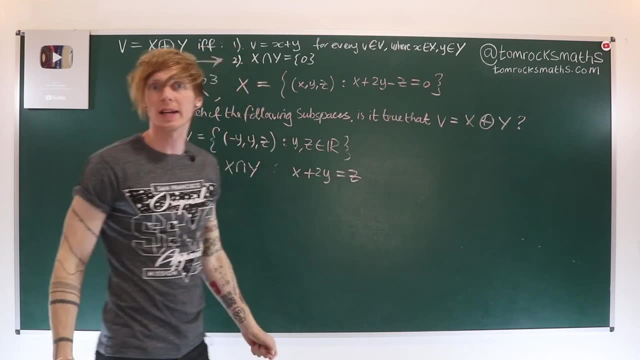 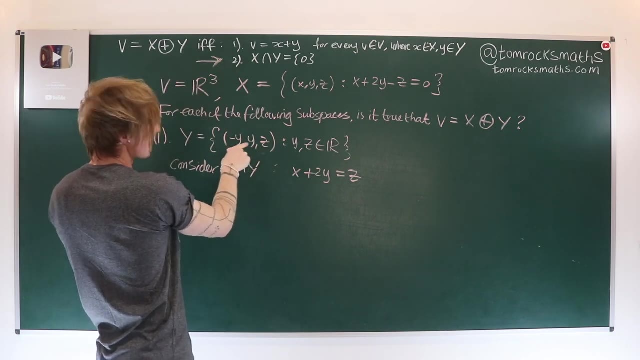 this form. So what that means then is we have: X plus 2Y is equal to Z, just taking that minus Z across. And then here we have: Z can be anything, and then the only restraint here really is this relationship between X and Y. So this is: 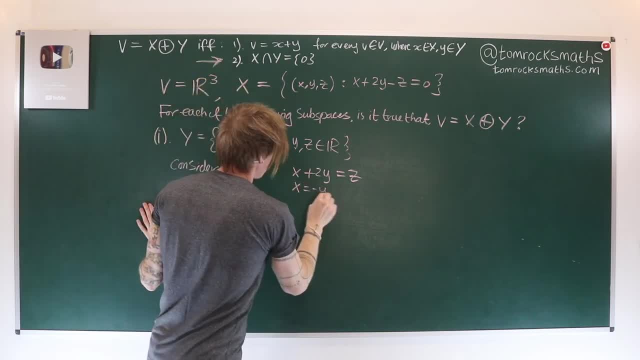 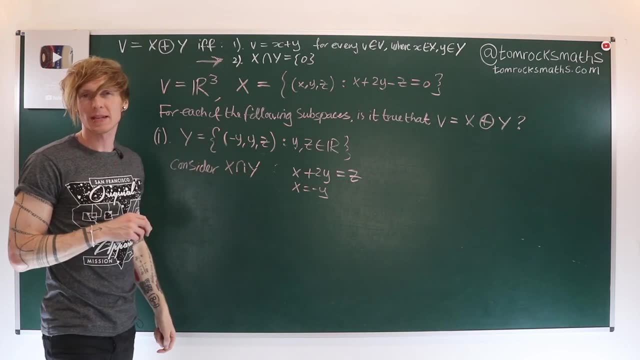 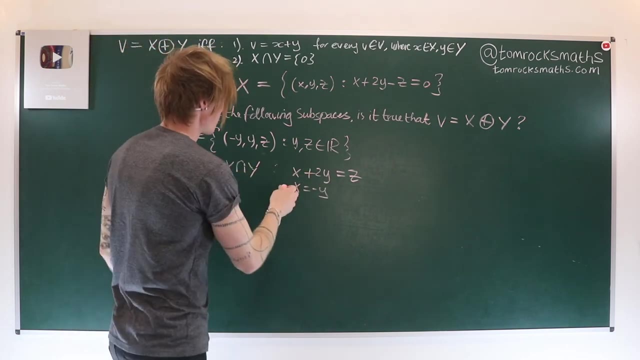 telling us that X must be minus Y, But Y and Z can be absolutely anything we want. so that's actually the only restriction we get from this particular subspace. So X plus 2Y is Z, but X is minus Y. so if we sub that one into here, then our top equation tells us: in fact: 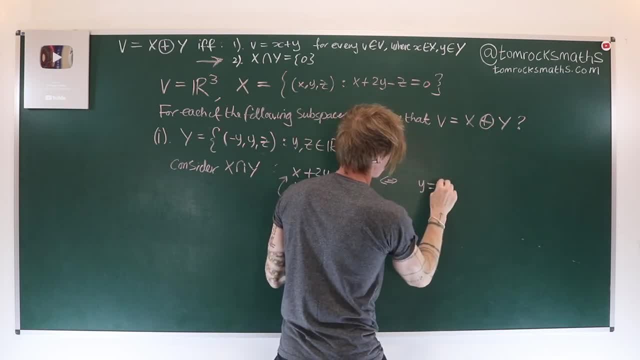 that Y is going to be equal to Z, and our bottom one tells us that Y is also minus X. So that's the only restriction we get from this particular subspace. So X plus 2Y is Z, but X is minus Y. 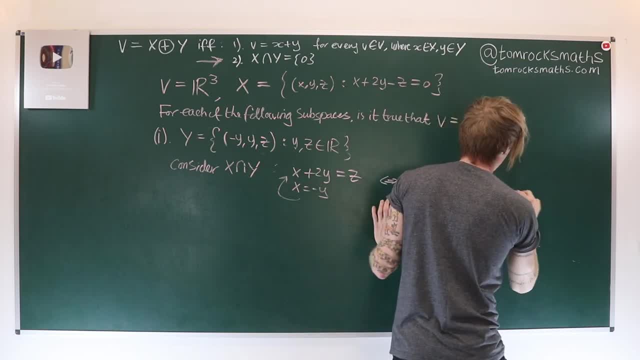 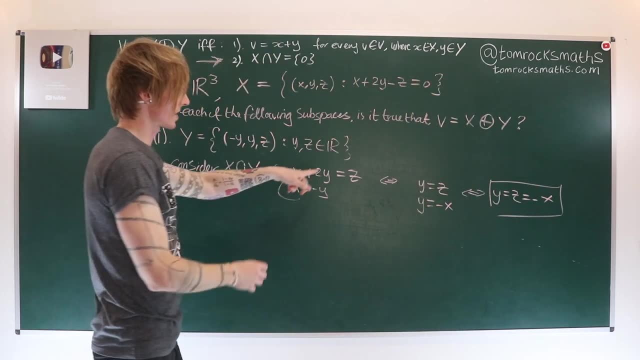 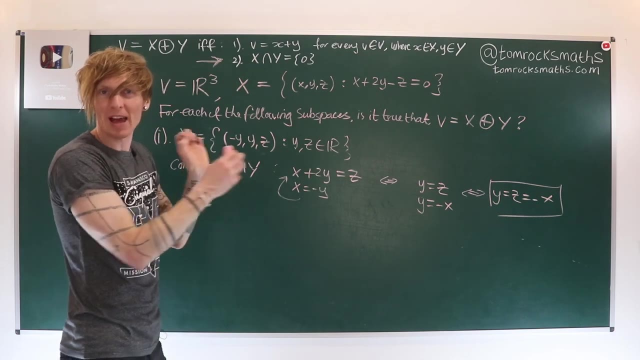 So, in other words, Y needs to be equal to Z, which needs to be equal to minus X. all in a box. So anything that satisfies these two equalities is going to belong to the intersection both X and Y at the same time. So I could say: well then, for example, if I take the vector 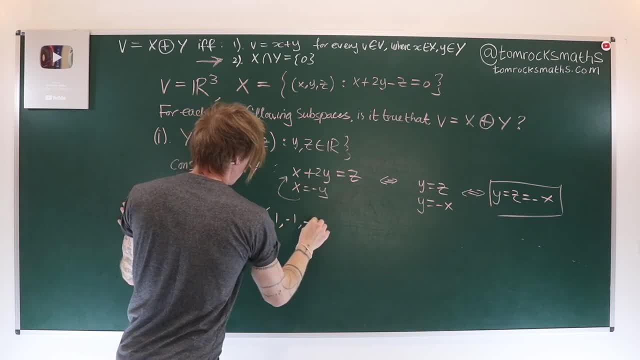 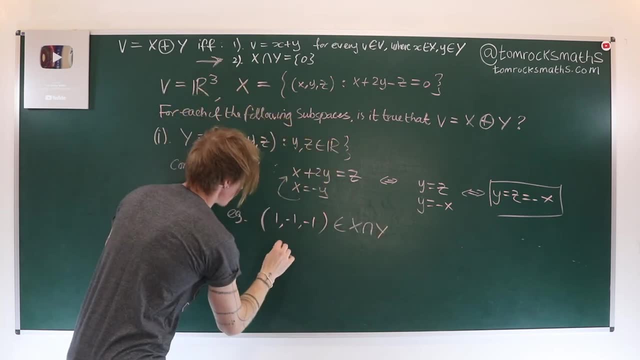 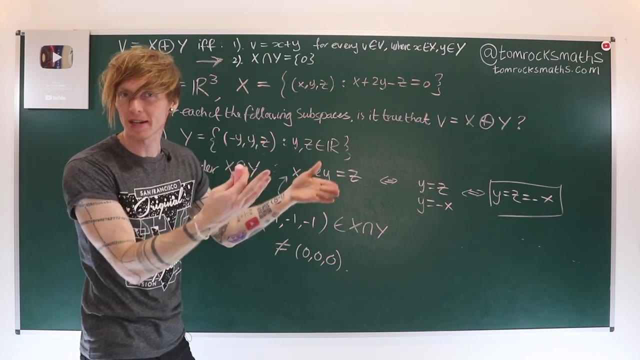 let's take X to be 1, then we've got minus 1 for Y, minus 1 for Z. Then I believe this is going to belong to the intersection and this is clearly not equal to 0. And of course, here 0 is the origin: 0, 0, 0, in this context of R3. 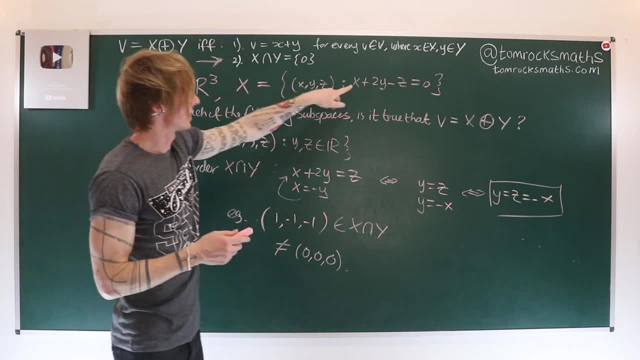 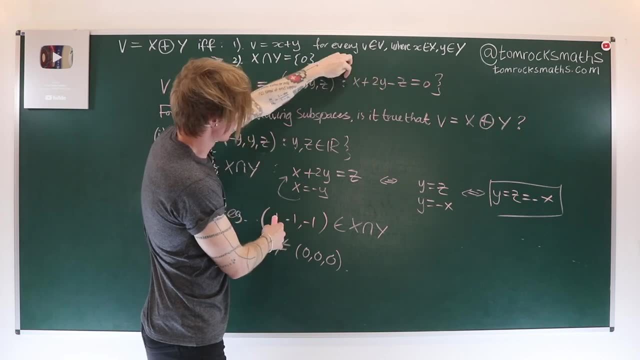 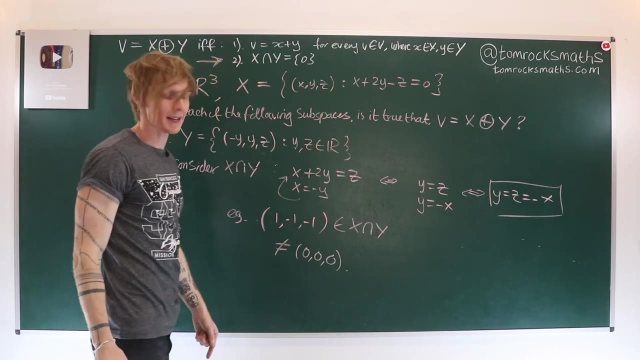 So let's just double check. does this vector satisfy this equation? So we've got 1, minus 2, so that gives us a minus 1, minus minus 1 gives us a plus 1, that gives us 0.. So this does indeed belong to X and also does it have this form. 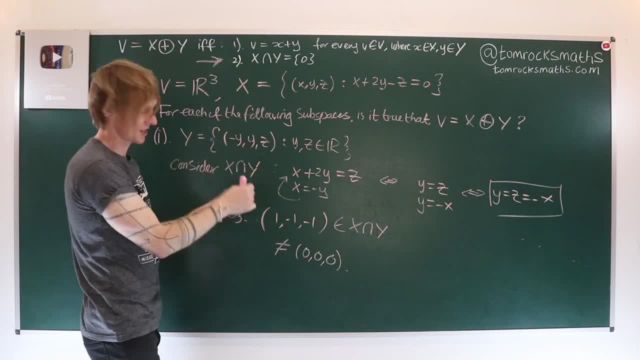 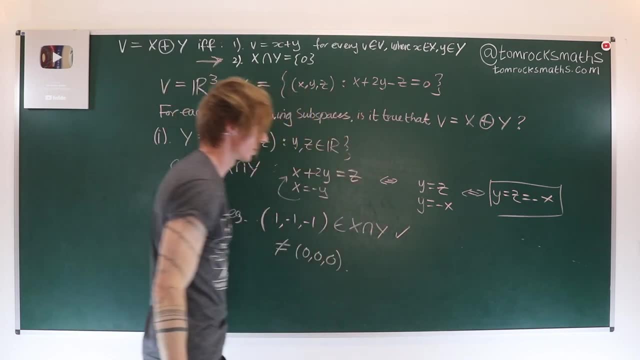 So we have Y, and Z can be anything, and then X. our first entry has to be the negative of the second entry, So it also satisfies that. So this is true, it does belong to the intersection and it is non-zero. 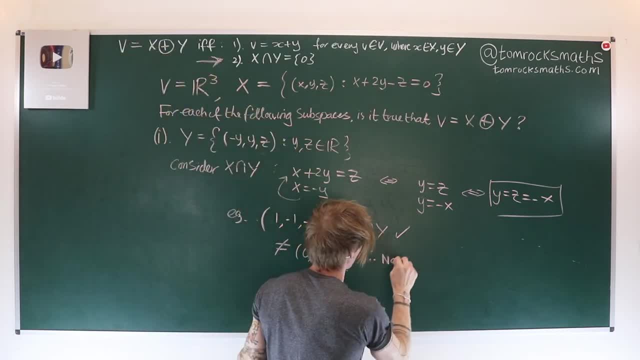 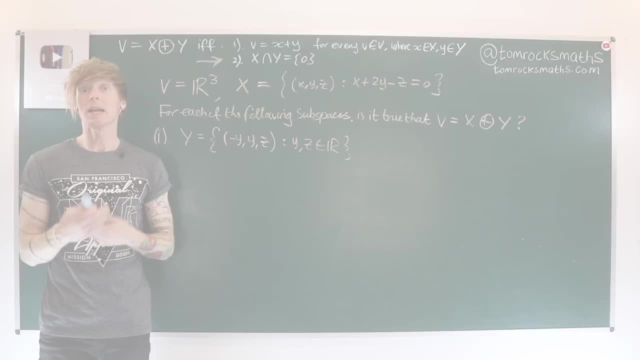 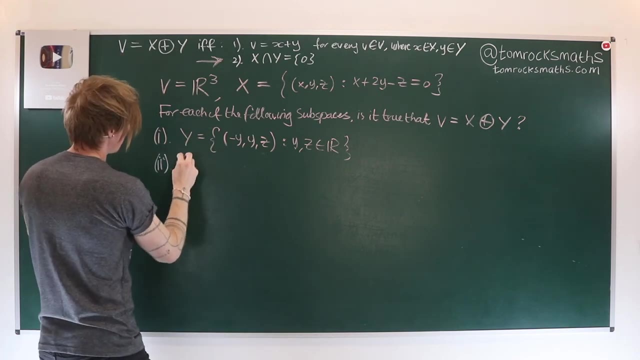 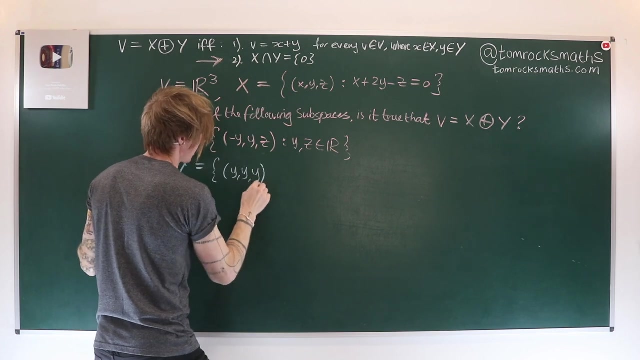 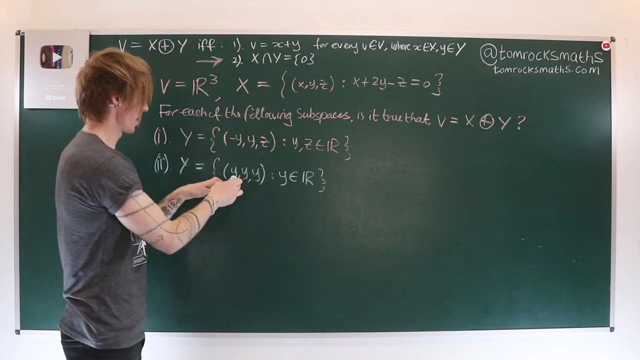 So therefore we can say: not a direct sum. Now let's look at our second example, which is going to be the subspace. Y is equal to Y, Y, Y, Where this is a real number. So in other words, we have to have the same value in the first, second and third position. 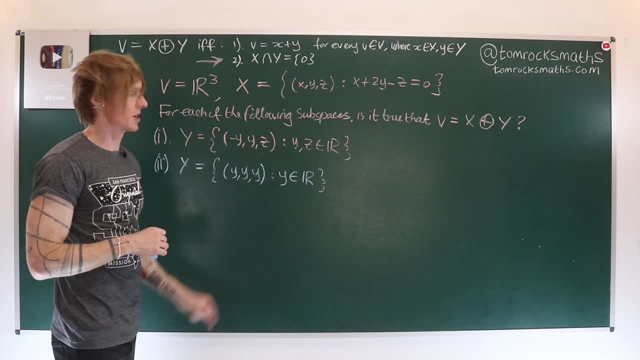 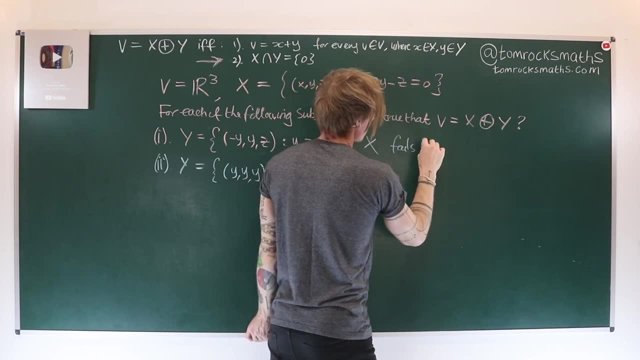 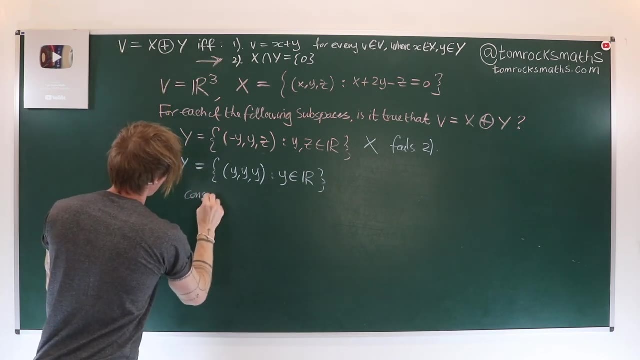 So, as before, we're going to consider the same value in the first, second and third position. So the second condition, because we saw this one failed, false fails, 2. Should have written that before, Okay, so let's again consider X. intersect Y. 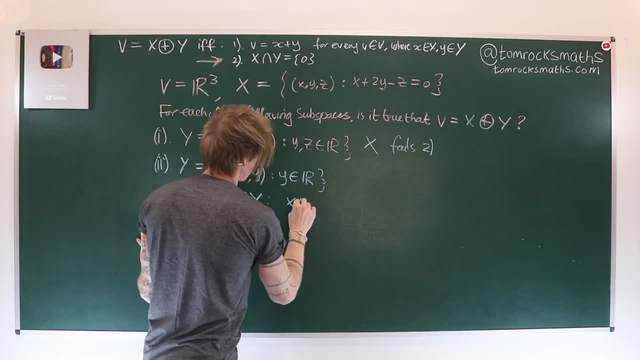 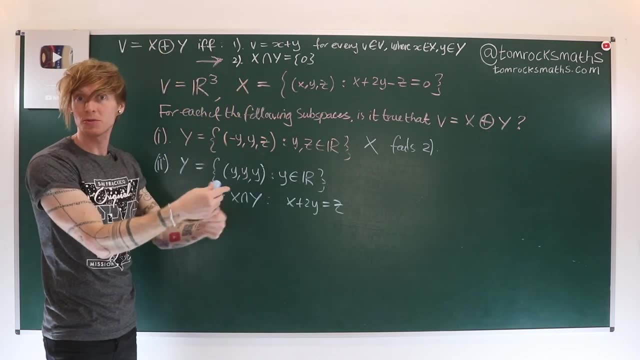 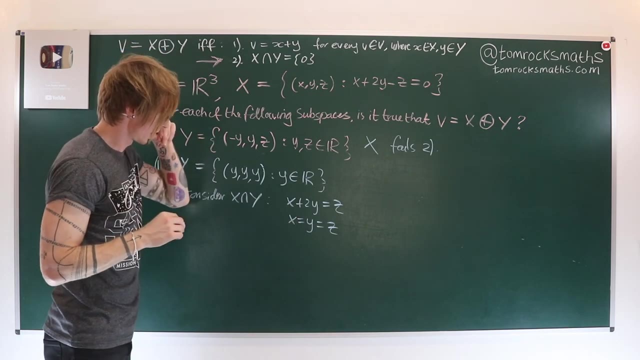 So we need: X plus 2Y is equal to Z, And we also need: according to this definition, X equals Y, So X equals Y equals Z. So in other words, we need X plus 2Y, but X is Y. 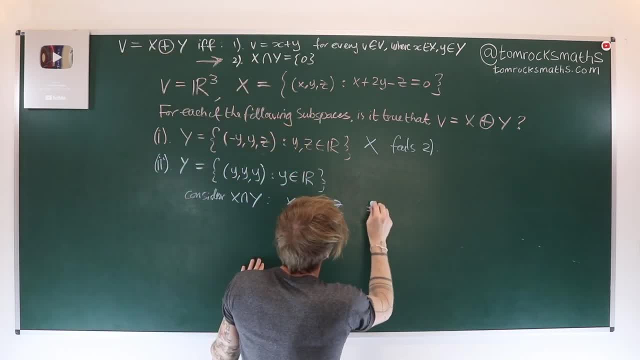 So we need: 3Y equals Z, but we also know that Y and Z are the same thing, So that's actually equivalent to saying that 3Z equals Z. ie, Z is zero And once we've got that, Z is zero. 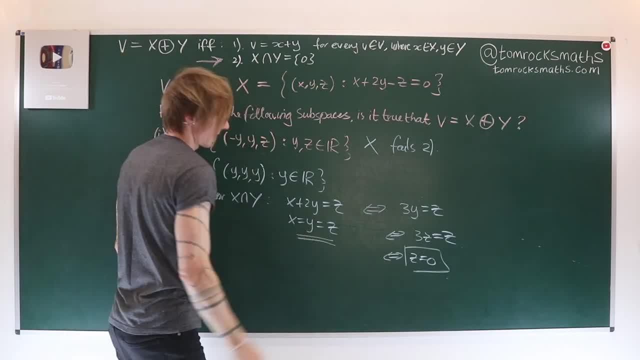 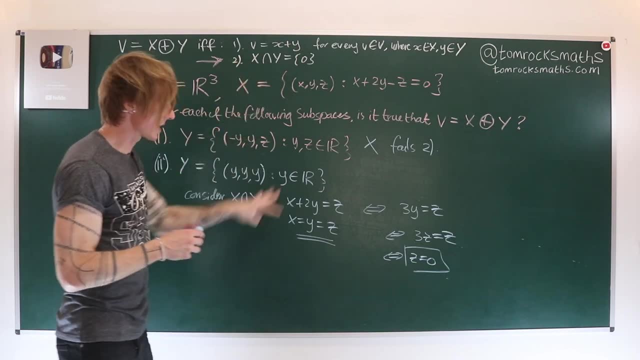 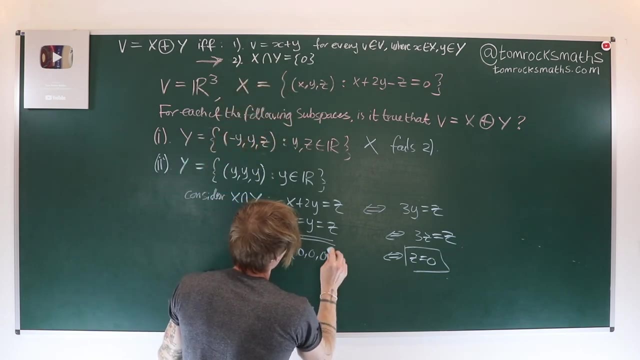 we can then see: from x equals y equals z, they're all equal to zero. So the only thing that's going to satisfy the intersection of x and y, these two vector spaces, is in fact going to be zero, zero. zero therefore belongs to the intersection and nothing else is going to satisfy these equations. 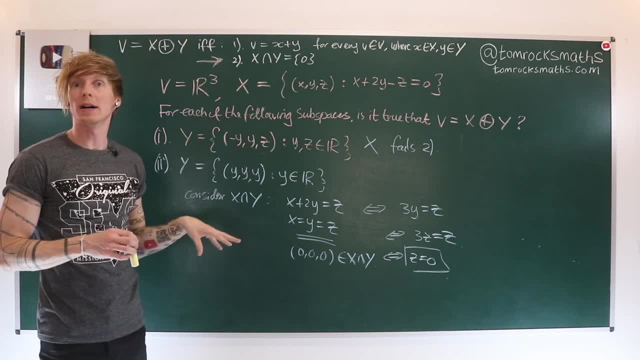 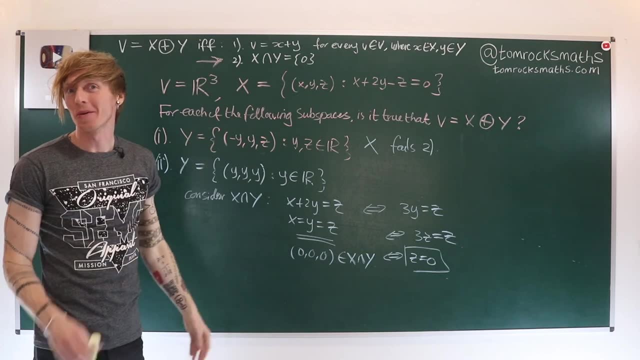 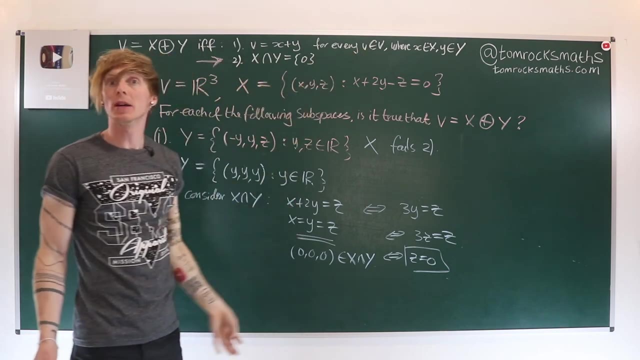 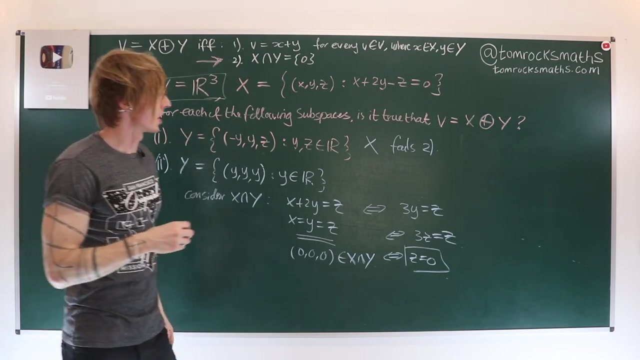 So now we know the intersection of x and y is indeed only the zero vector. we are actually going to have to check condition one. Now. what this is saying is for any general vector v belonging to our larger space. so here v is 3D coordinate space, R cubed. so really, 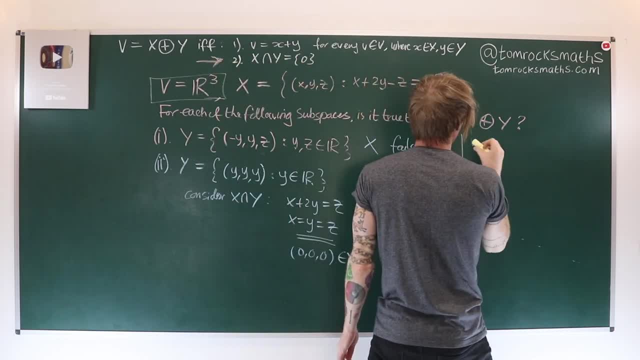 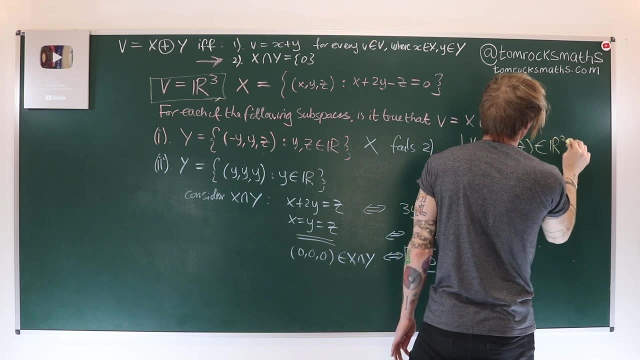 what this is saying is: our vector v is equal to v times 3d r squared, and this is going to specify how are we about to get c and d in a row. Now we know the intersection of x and y is, indeed only is going to be x, y, z belonging to R cubed, And we need to rewrite this as some piece. 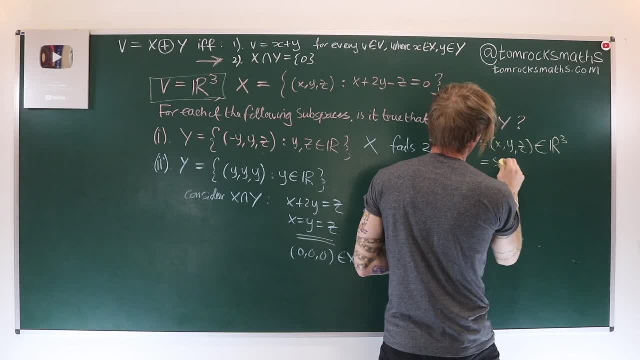 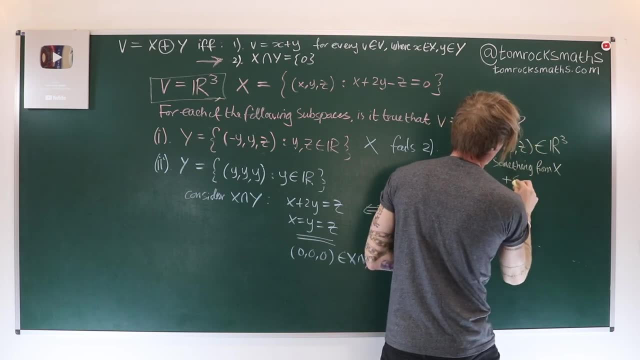 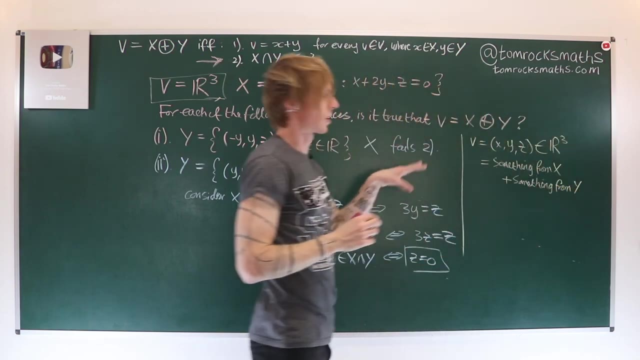 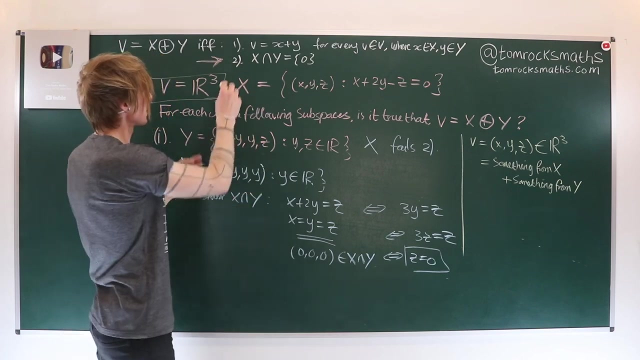 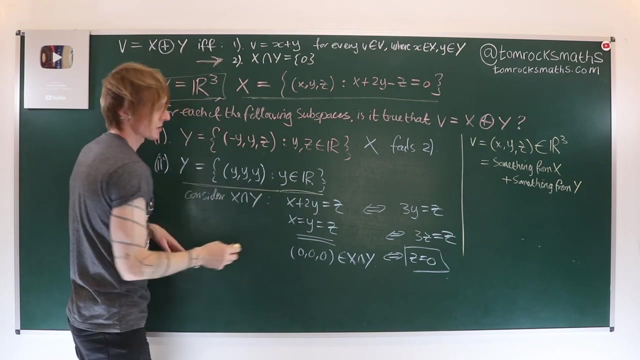 from capital X. so equals something from capital X plus something from capital Y. So our goal here is to take the most general point we can, so an x, y, z coordinate and rewrite it as something that belongs to this plus something that belongs to this. 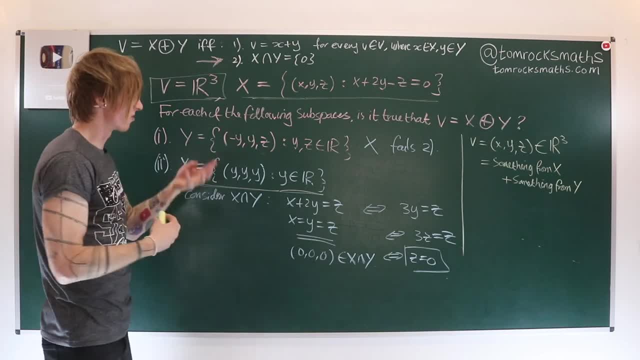 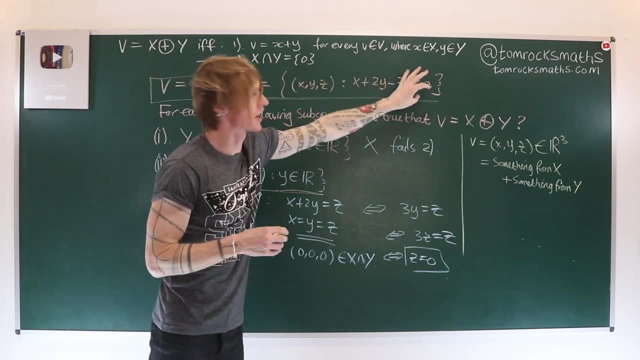 So, since we want to be as general as possible, really we need to know the basis of both of these sets, because anything in X is going to be written as a linear combination of its basis vectors And similarly, anything in Y is going to be written as a linear combination of its basis. 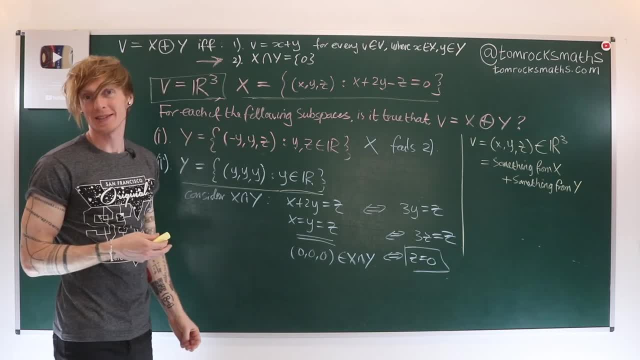 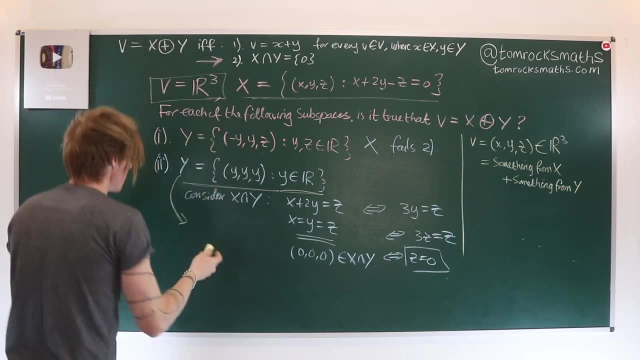 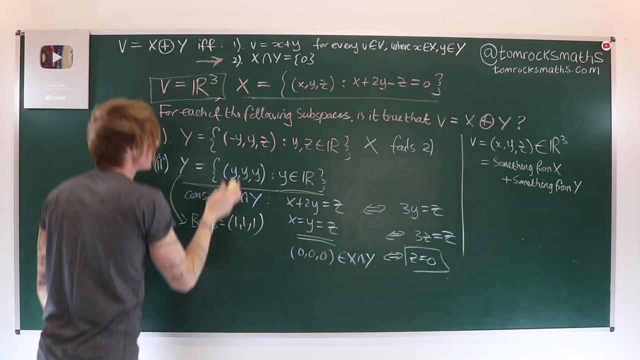 vectors. So Y is actually a little bit easier because again, x, y and z, the three entries are all the same. So the basis here is simply the vector 1,, 1, 1, because anything in this set is just 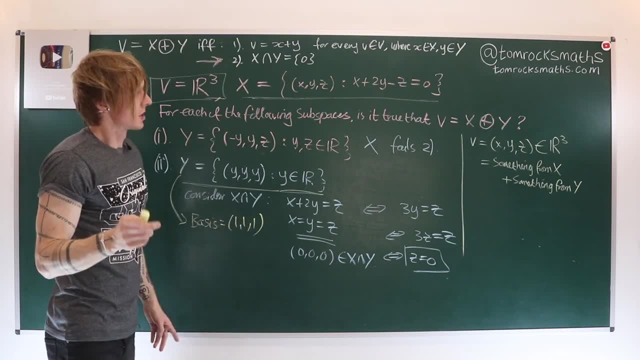 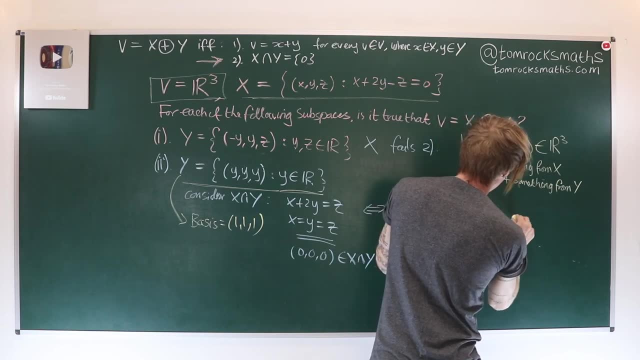 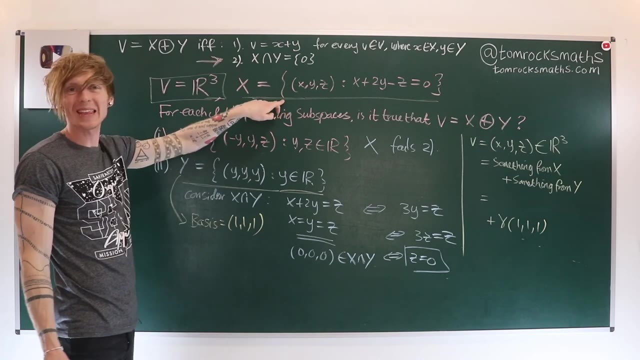 simply a multiple of this vector, So something from Y. that's quite easy. So we don't know what X looks like yet. But the thing in Y is going to be gamma, Gamma times 1, 1, 1.. Now for the thing in X. we need to know what the basis of this is going to be. 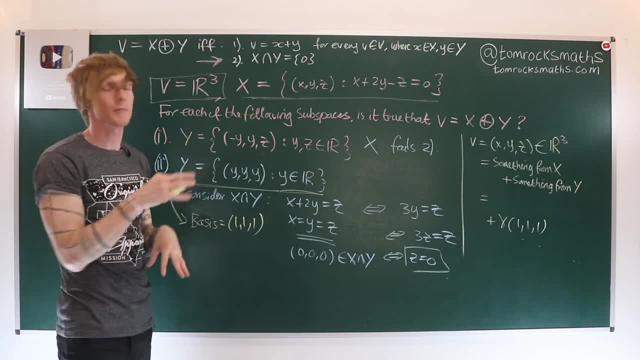 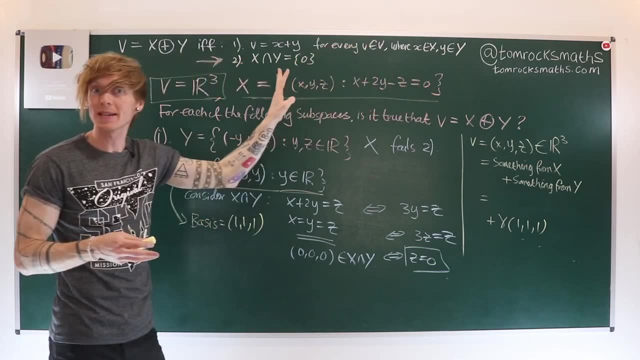 So we saw something similar to this in the previous video, when we were looking at the dimension formula and we had some examples where you needed to work out the dimension of a subspace, and we did that by working out the basis and then counting the number. 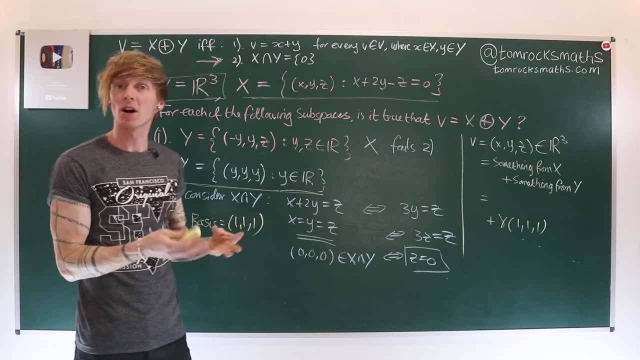 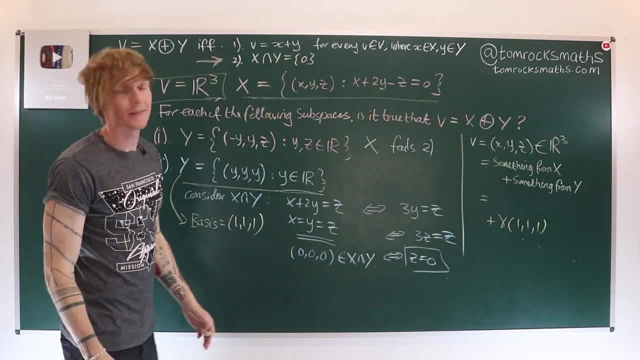 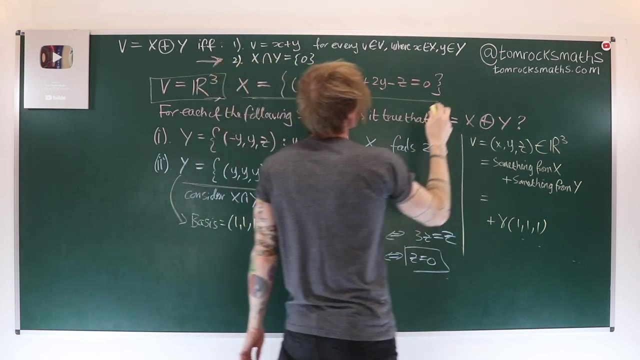 of basis vectors. So here we want to do a similar thing, but rather than just counting them, we actually want to use them to construct our general point in the space of E. So we have to have that X plus 2Y minus z is 0.. 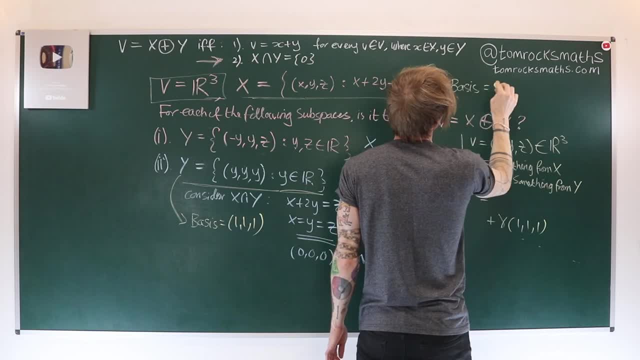 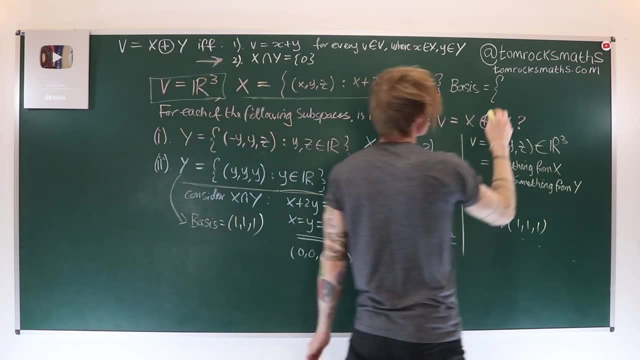 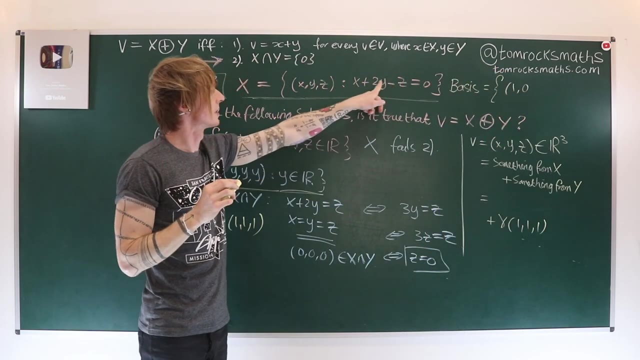 So let's think about what the basis has to be here. So as a starting point, let's suppose I fix X to be 1.. So if X is 1, let's make Y 0. And then I now need to have: 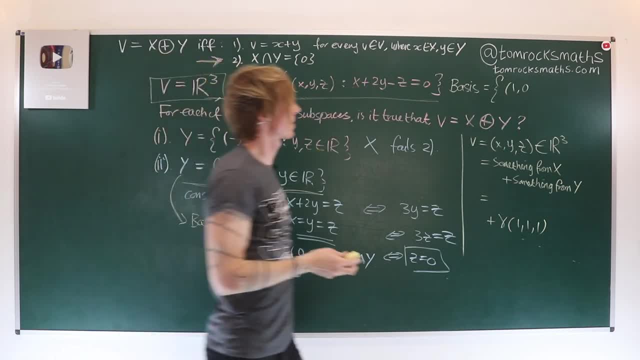 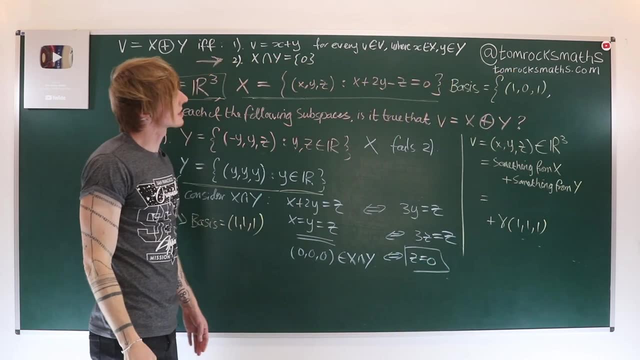 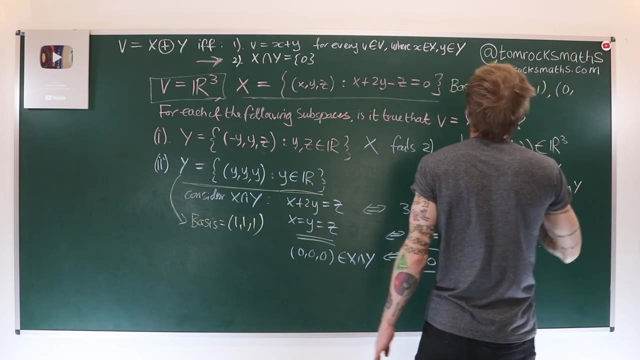 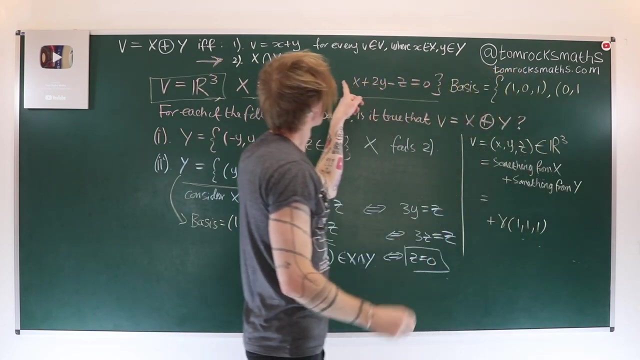 X equal to z in order to satisfy this expression, so that would be a 1.. And then if I did something similar, and now let's suppose we set X to be 0,, then what is this going to tell me? So if I pick Y to be 1, for example, then I've now got 0 plus 2 minus z has to be 0. 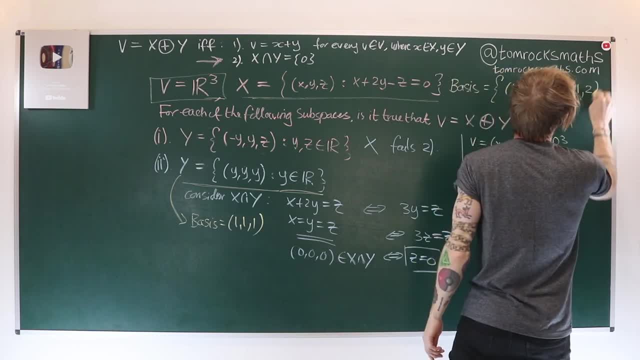 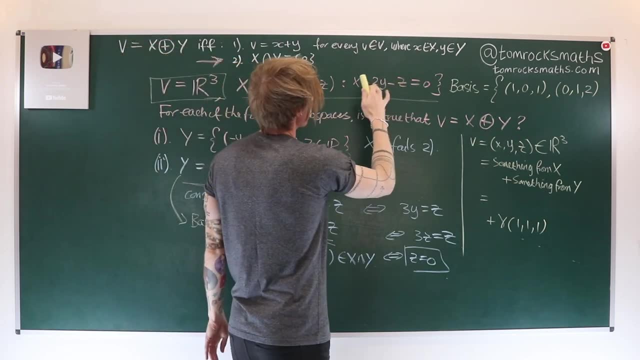 So z has to be 2.. So I could have 0,, 1, 2.. Now, continuing this way, I could also set z to be 0. But if I set z to be 0, I then have X plus 2Y needs to be 0. 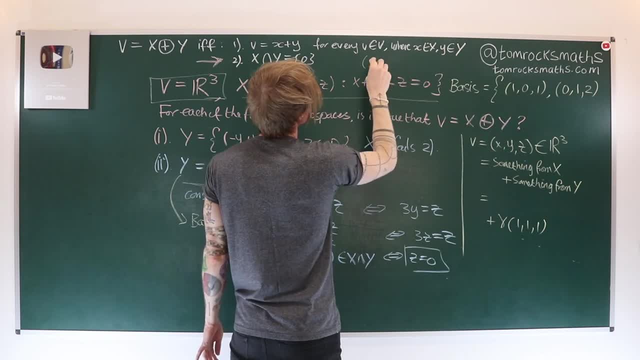 So I would end up with something like: what would I get? So if Y was 1,, z was 0, then X would now have to be minus 2.. But looking at what I've got already, I think I can actually. 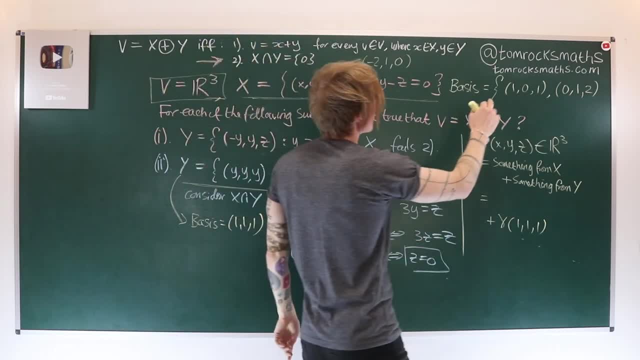 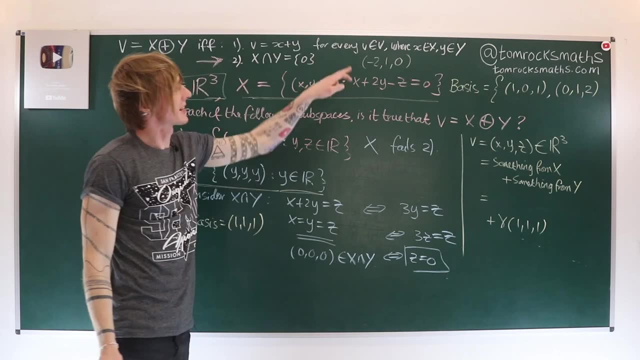 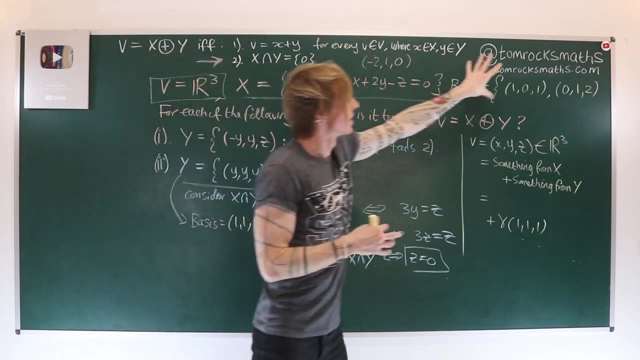 get this vector, Because if I take minus 2 lots of the first one and add that to the second one, I'm actually going to get exactly this vector. So this wouldn't be an addition, wouldn't be another linearly independent vector to 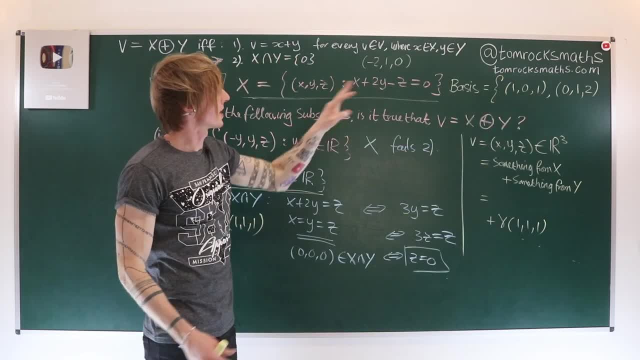 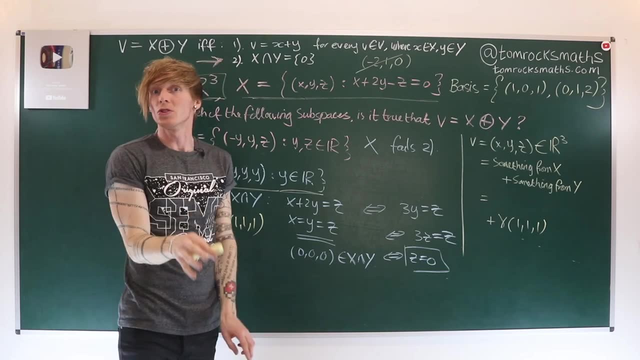 add, It would actually make the set linearly dependent. So I actually think that that one isn't needed And this, I believe, is going to be my answer, To be my basis. Now, of course, you should all check this. 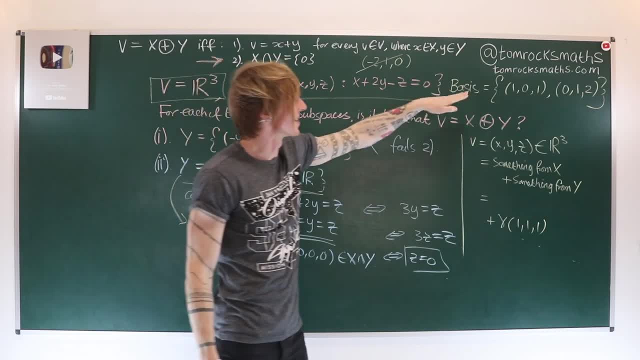 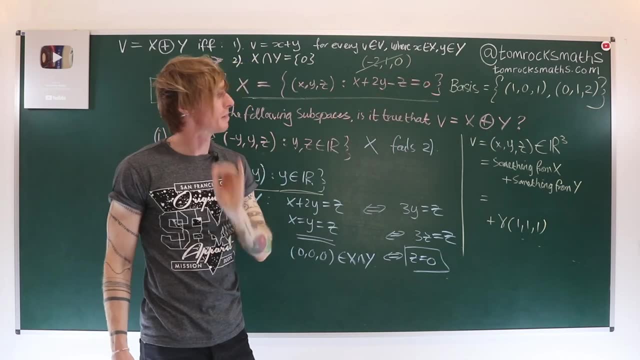 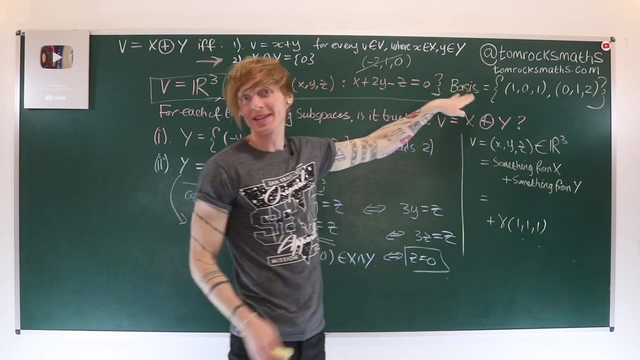 I am just telling you this is correct, without, of course, checking that these two vectors both span this space and are themselves linearly independent, But I believe this should be correct, So I would recommend that as an exercise to check. this is, in fact, the basis of our space. 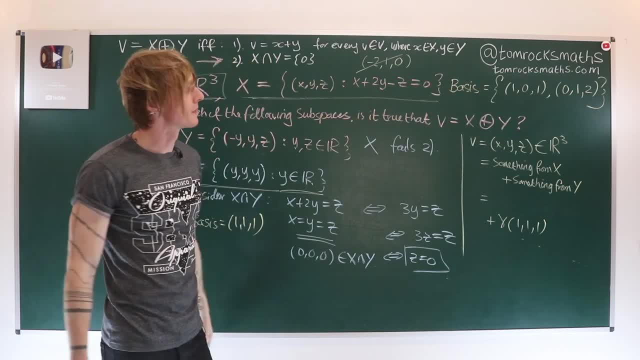 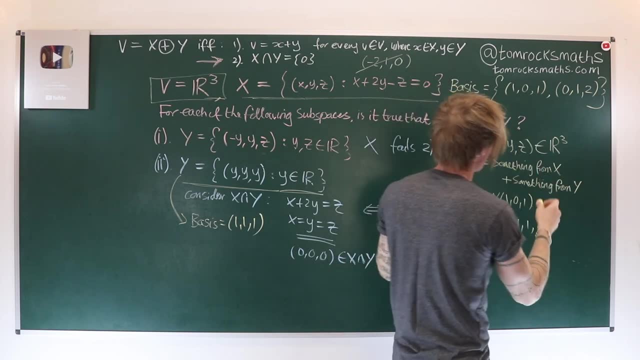 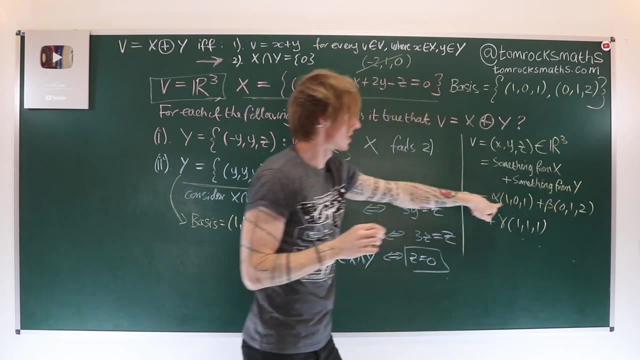 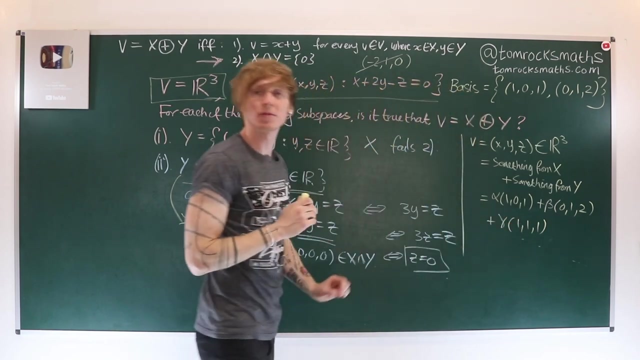 X, But taking that as true for now. we therefore can say: we need alpha, Alpha times, the first piece, plus beta times, the second piece, And then that gives us something, the most general possible thing in our space X, And this piece gives us the most general possible piece from our space Y, over here. 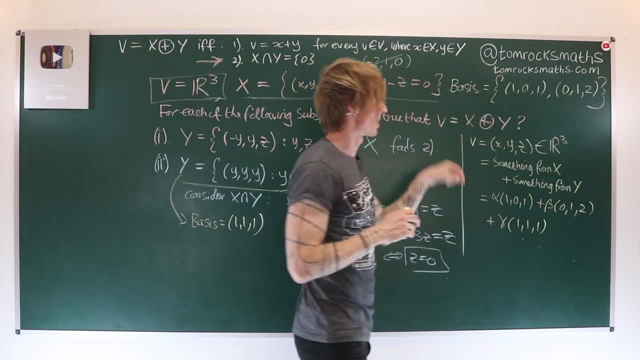 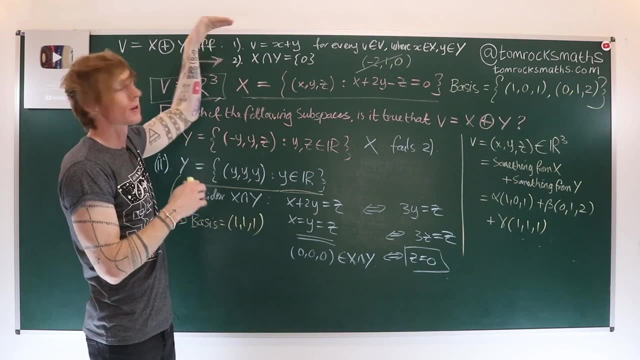 So now we just have to solve for alpha, beta and gamma in terms of X, Y and Z, And hopefully we can get a valid solution. If we can get a solution, then we can conclude that one holds and therefore we have a direct sum. 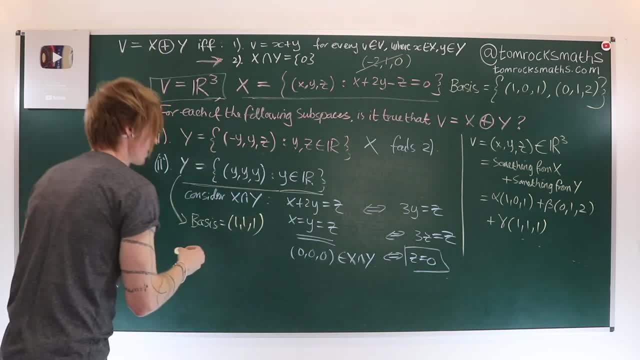 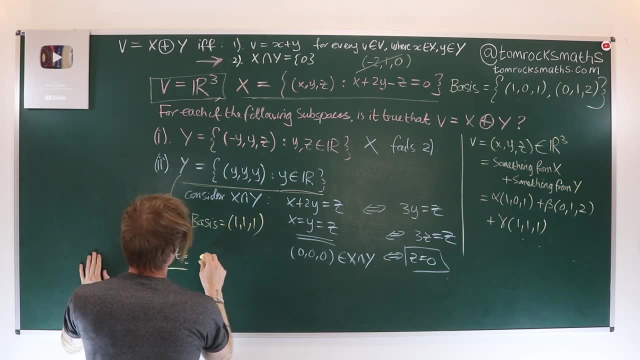 So let's do the algebra. If we begin with the first coordinate down here, What have we got over there? We've got: alpha plus gamma has to be X, So X equals alpha plus gamma. From our second coordinate we have Y has to be equal to X. 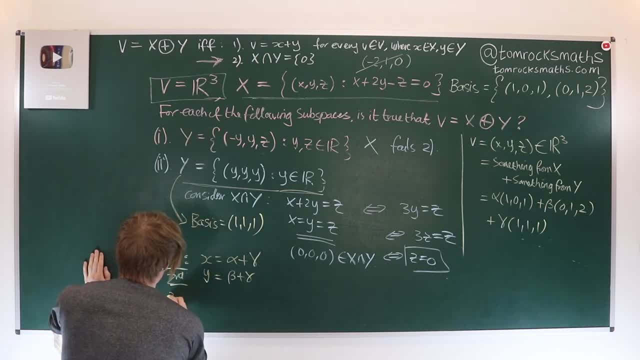 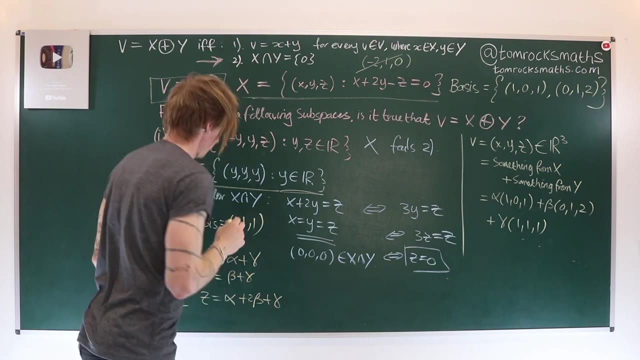 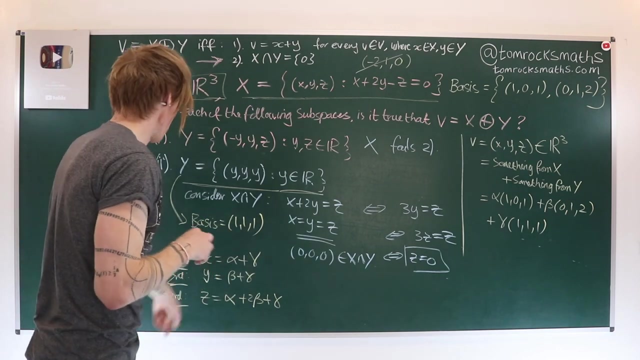 To beta plus gamma and from our third coordinate we are going to get that Z is equal to alpha plus two beta plus gamma. Okay, so remember, we want to solve alpha, beta and gamma here in terms of X, Y and Z. So let's take the middle one and say: beta is there. 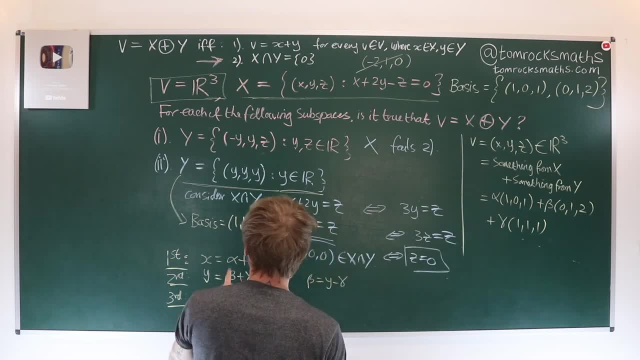 Beta is therefore equal to Y minus gamma. Let's plug that in the top, which will then tell us that X is equal to alpha plus gamma. So I can rearrange that to get alpha in terms of gamma. So alpha is equal to X minus gamma. 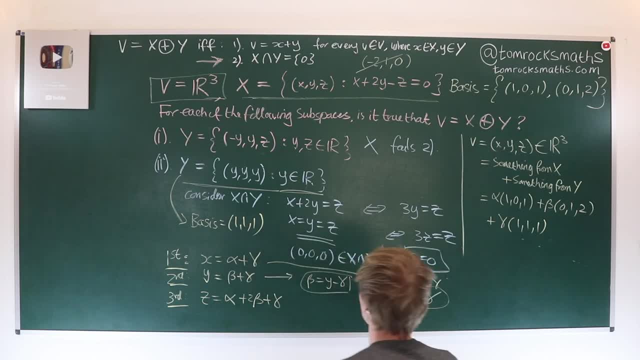 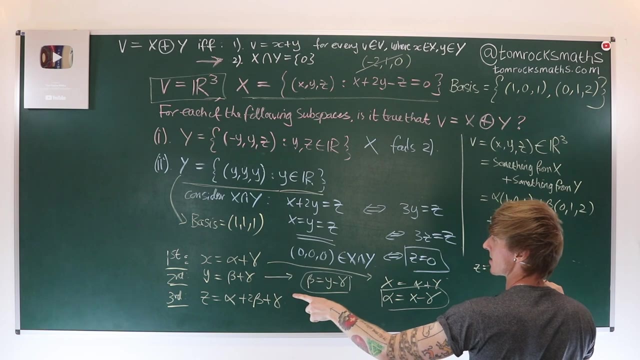 So now I've got alpha in terms of gamma, beta in terms of gamma, So let's plug those two into the third one And I'm going to get. Z is equal to alpha, which is X minus gamma plus two beta, plus two Y minus two gamma, and then plus a gamma. 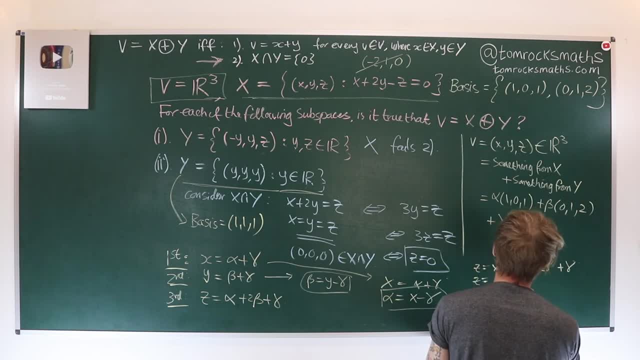 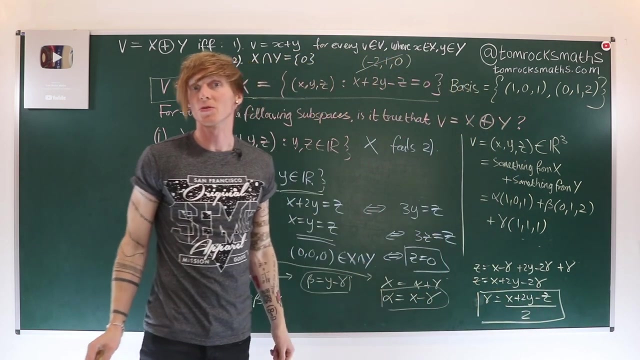 Okay, so I've got Z equals X minus gamma, plus gamma minus two gamma. So X plus two Y minus two gamma. So that tells me that two gamma is X plus two Y minus two gamma. So I've got it y minus z. so gamma divided by 2 is that. So I believe that gamma is going to be x plus 2y. 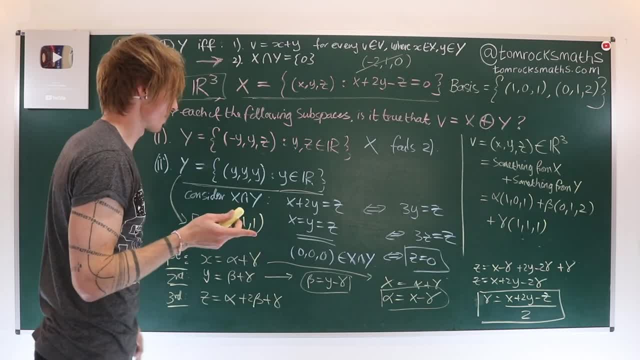 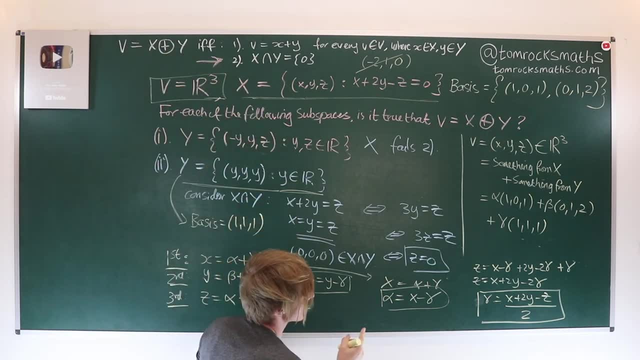 minus z over 2.. That's going to now give me beta. so that means from here, beta is now y minus that, so that's going to be 2y minus x minus 2y plus z all over 2, so that's going to cancel out the y's. 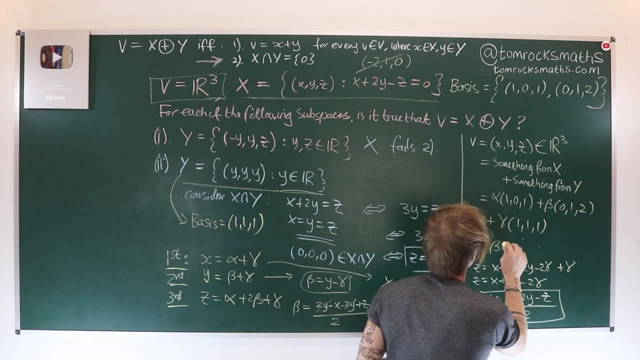 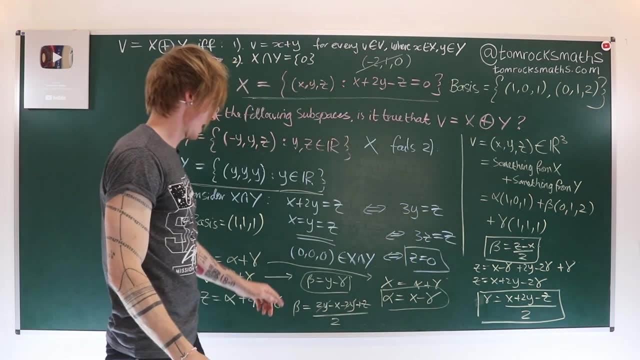 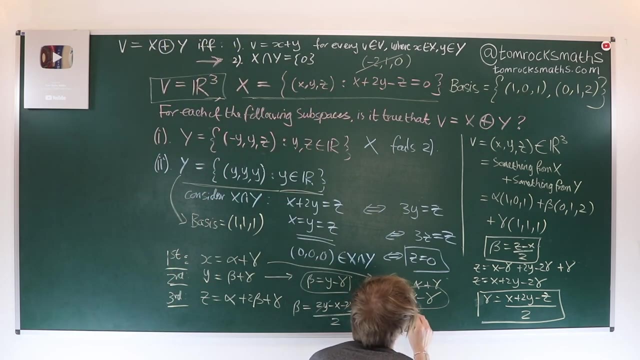 So beta is z minus x over 2,. beta is z minus x over 2, put that over there and then finally I should be able to now get: alpha is x minus gamma, so that's equal to 2x minus x over 2.. 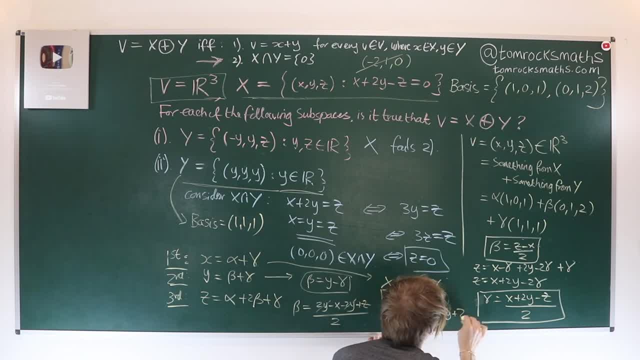 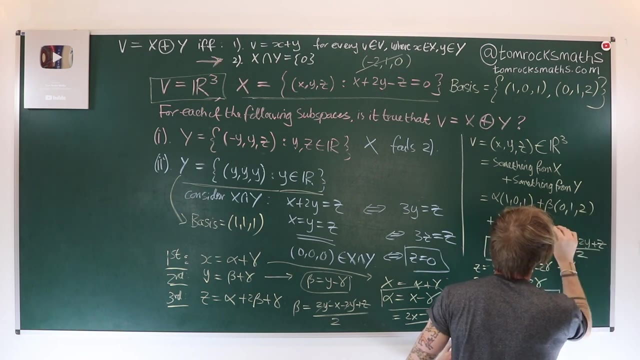 x minus x minus 2y plus z and that's all over 2, so it's x minus 2y plus z over 2.. Okay so I believe- and I'm sure all of you watching this will check my working- 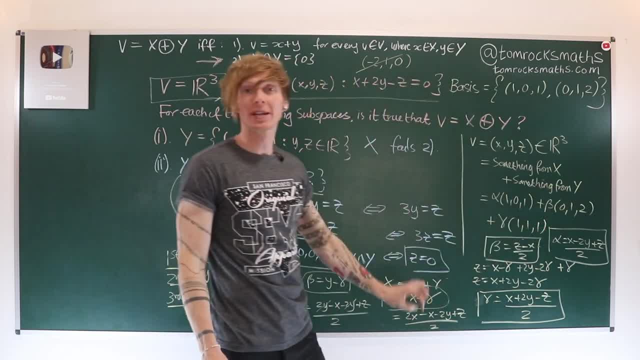 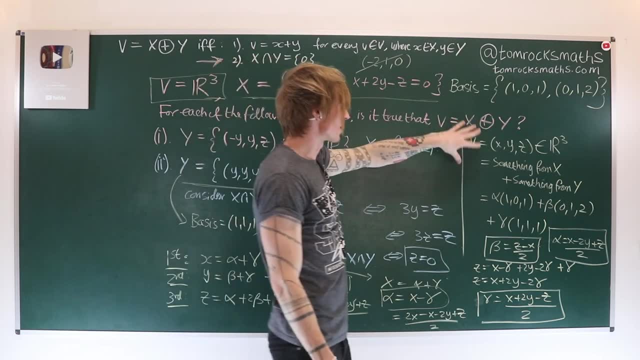 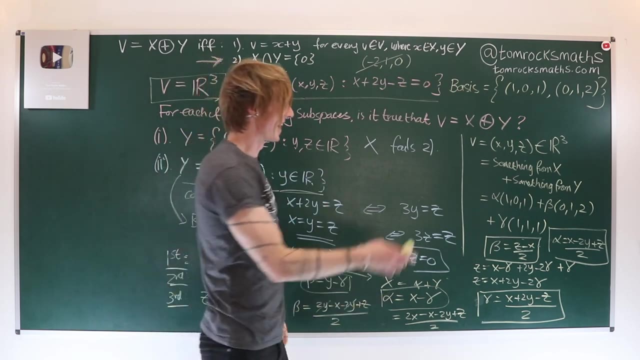 I believe alpha, beta and gamma, as written here, should indeed be valid solutions to substitute in- and again, please do check this for me- and we can see that any general vector- x, y, z- which is a general point in R3, can indeed be written as alpha. 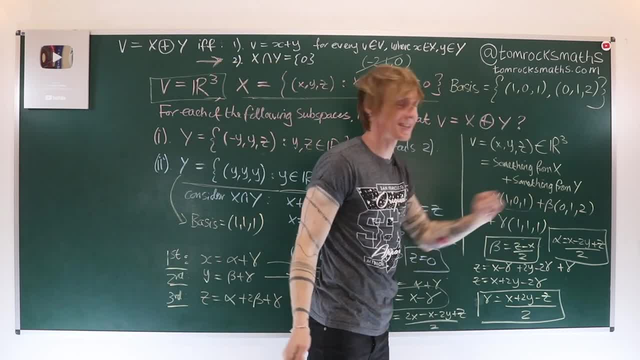 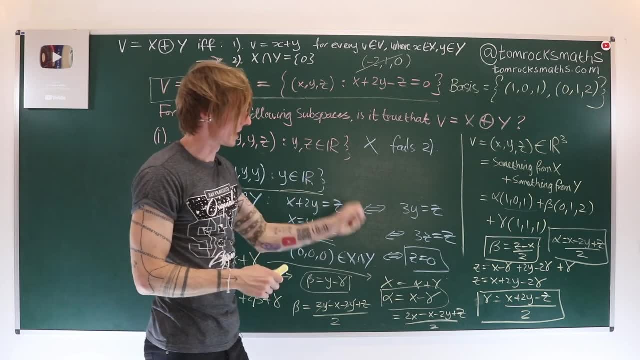 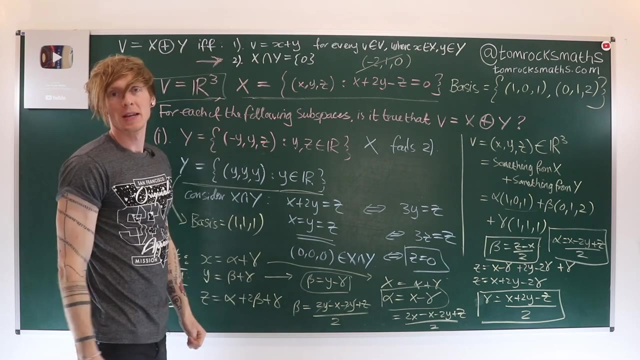 of the first basis vector of x plus beta times the second basis vector in x. but importantly, those two added together are something in x plus gamma, lots down here of 1, 1, 1, 1, which is something that belongs to y. So it was hard work, which is why I said we usually 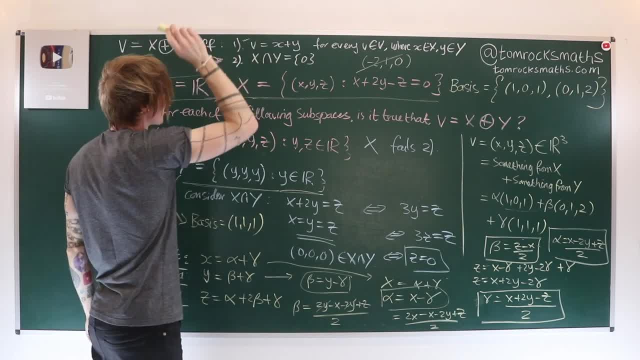 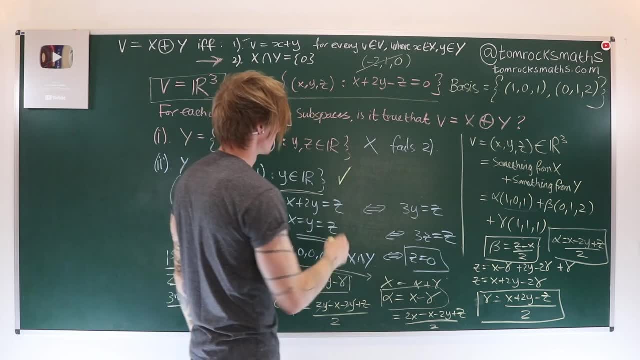 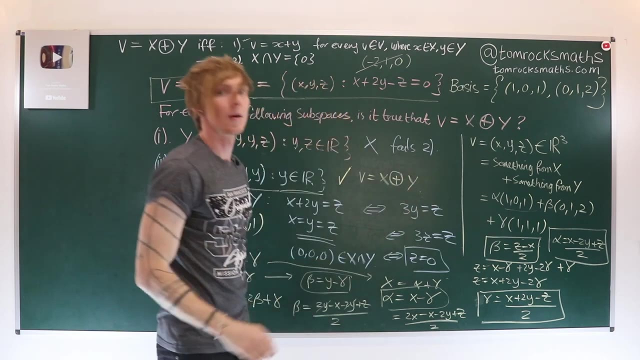 start with number 2, but we've also shown here the number 1 holds and therefore we can conclude going back to our original question. this is true. so yes, is a direct sum. so v is indeed x direct sum y. Our third and final example is going to be the following subspace: 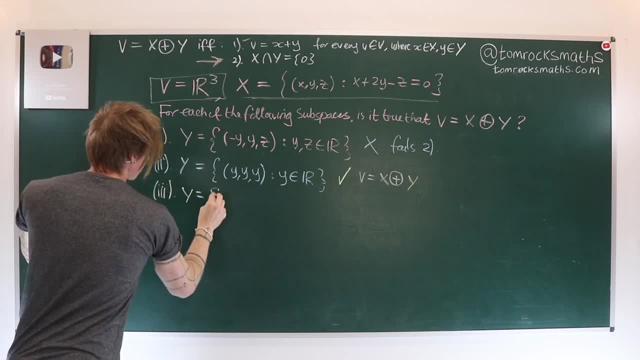 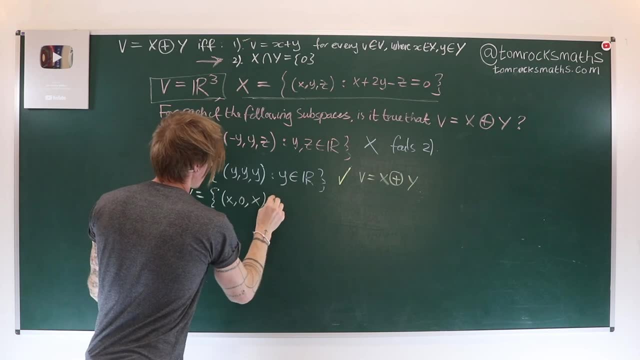 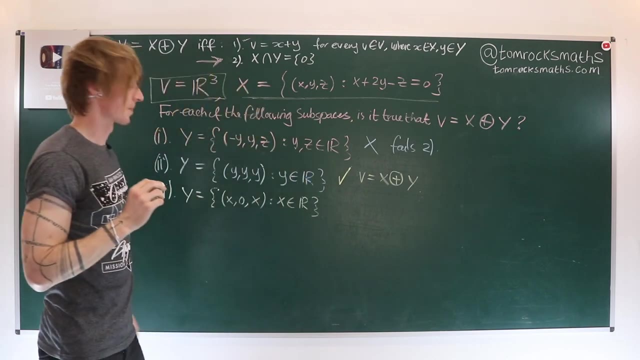 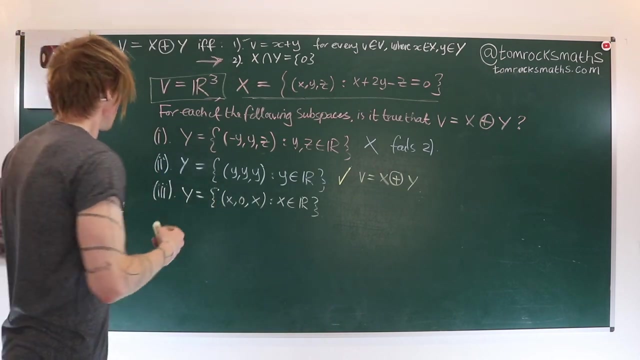 So y is equal to a triple vector where the first entry, x, is the same as the third entry and the y has to be 0, so where x can be any real number. So we proceed in exactly the same way as with the previous two examples. We are going to consider number 2, so consider the intersection. 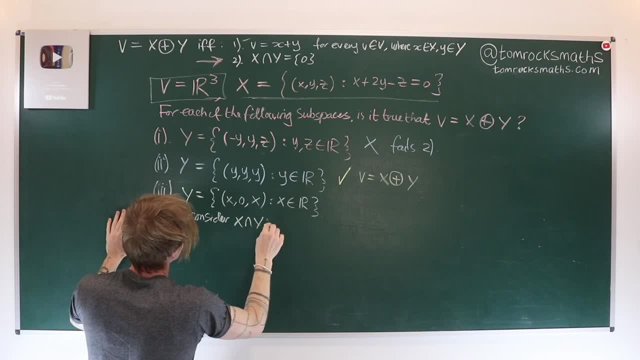 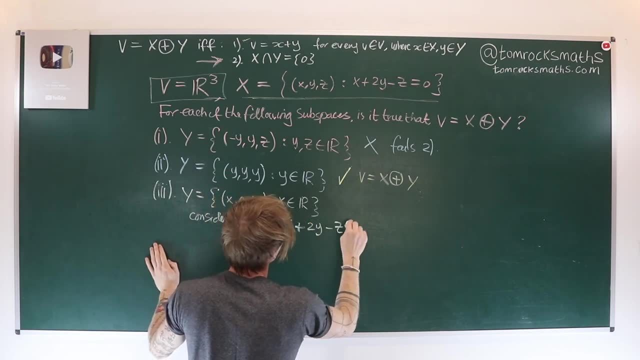 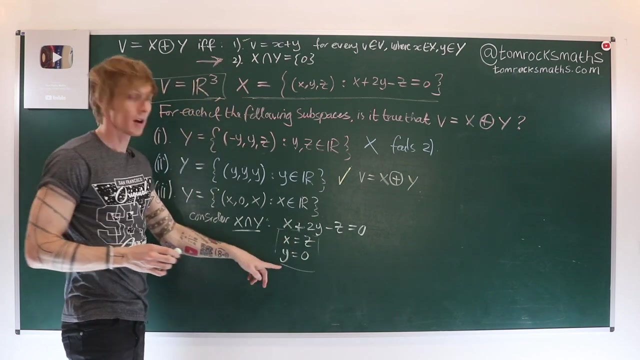 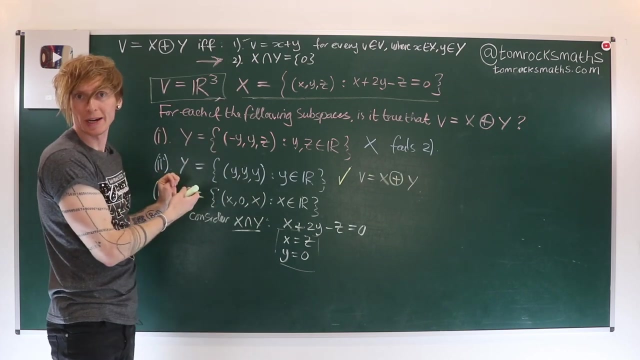 first Consider x, intersect y. So we need x plus 2y minus z must be 0 for x, and then to be in y we need x is equal to z and y must actually be 0. So these two conditions here are both derived from this particular form of all vectors belonging to our third subspace, y. 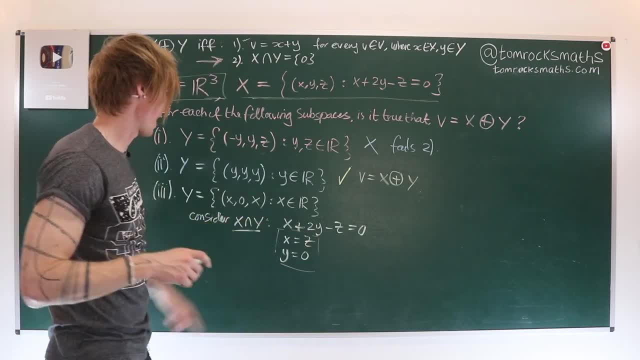 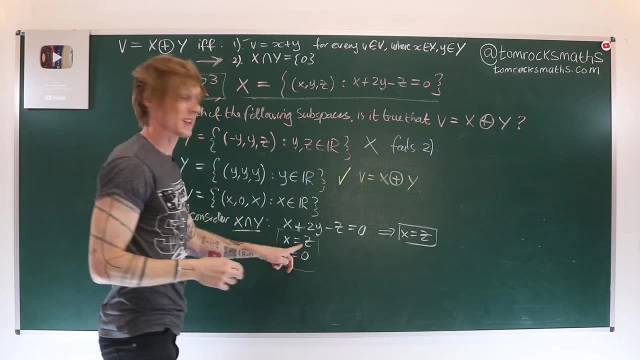 So if we substitute in: y is 0, then we get from the top line. this actually just becomes x equals z. So we have x equals z, x equals z again and y equals 0. But at no point do we require x and z. 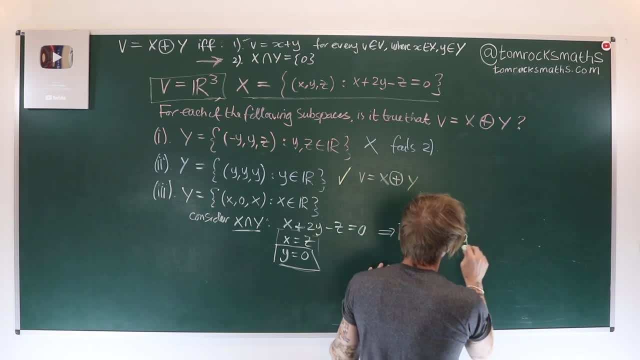 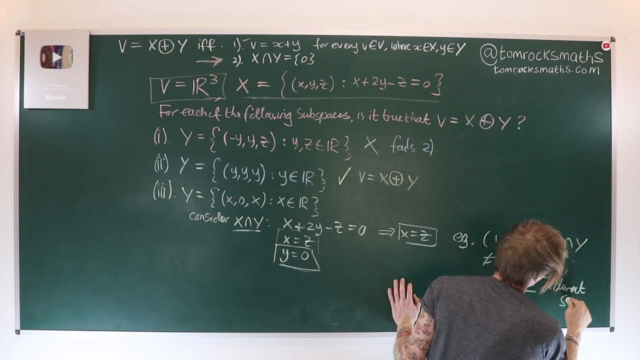 to be 0. So here- fortunately this is a quick one- We can just say: eg 101, I believe, will belong to the intersection of y and z, of x and y, which of course is not zero, not equal to zero, zero, zero, therefore not a direct sum. 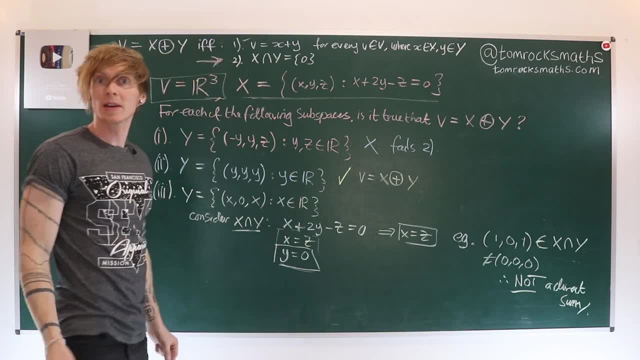 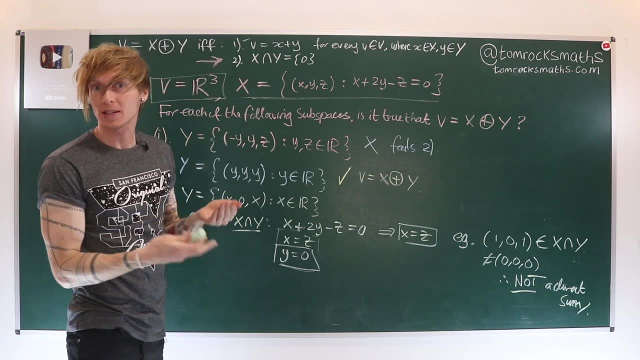 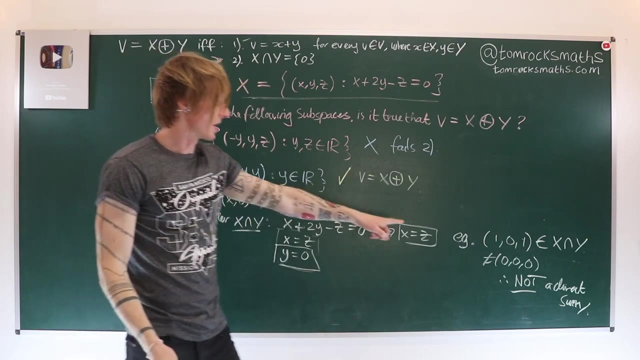 And we can very quickly check that that does indeed belong to both x and y. It clearly has this form: one zero one satisfies the requirement to be in the vector space y, and also we can see that one plus zero minus one is indeed zero. So this is in fact going to be in the intersection.